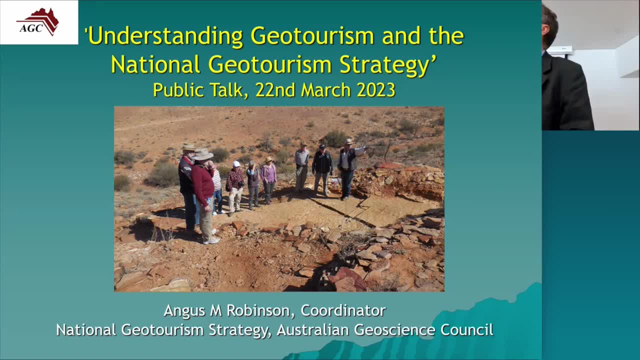 respects to the people, cultures and elders, past and present, And, of course, acknowledge any Aboriginal and Torres Strait Islander people present in the seminar today. Thanks everybody for joining us Today's seminar. the topic is Understanding Geotourism and. 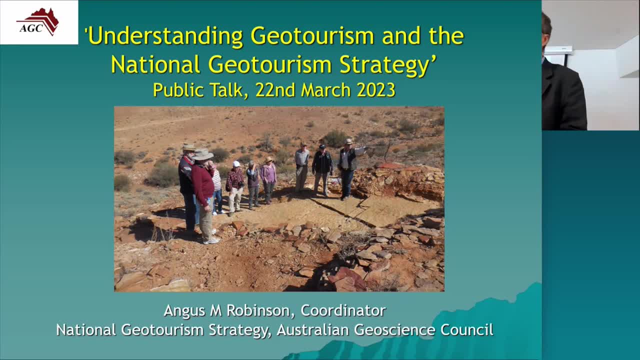 the National Geotourism Strategy. Our presenter is Angus. In a nutshell, Angus is going to be talking about how, by focusing on geology and geomorphology, as well as ecology and culture arising from these geological characteristics, considerable value can be added to nature-based tourism. 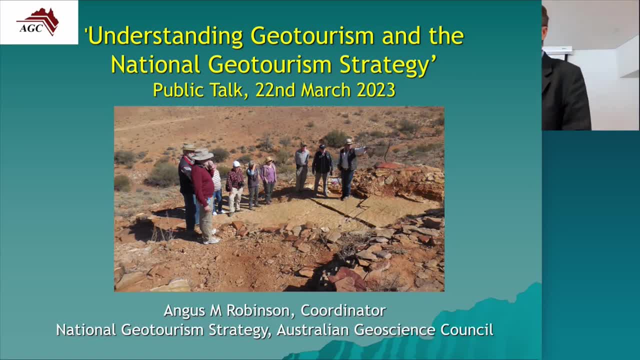 and Aboriginal tourism through the National Geotourism Strategy. Angus is an exploration geologist by profession and training. He's currently engaged in ecotourism and geotourism activities and serves in a pro bono capacity as coordinator of the national geotourism strategy for the australian geoscience council incorporated. 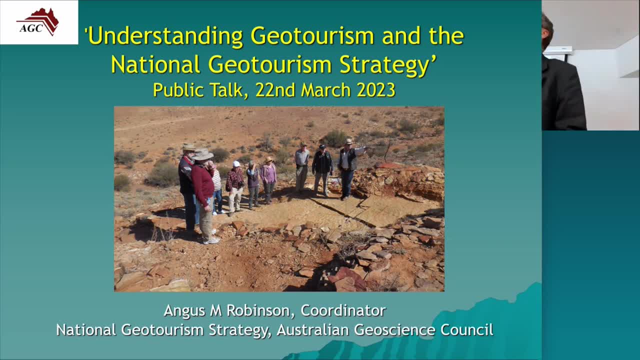 and i understand from my readings as i went through it last night, i think this is that's the, the peak body for some eight, eight of the national society. so so it's a peak body that's representing lots of our professional societies. uh, he's in that role as a pro bono capacity, uh. 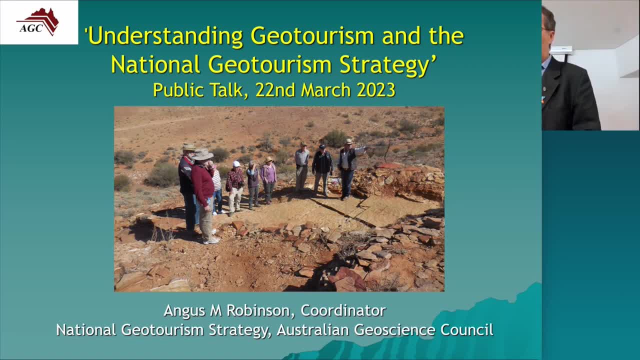 and this is follows his role as the inaugural chair of the geotourism standing committee of the geological society of australia, a long-standing member of the australian institute of mining and metallurgy, and also a member of the management committee of the social environmental society, as well as the heritage committee, um, over the past 30 years. 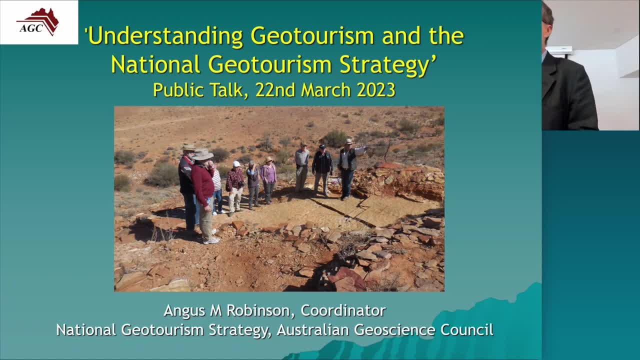 angus has been engaged in leadership roles relating to technology diffusions through the warren center of advanced engineering at the university of sydney, technology park development and as the chief executive of a major manufacturing industry association. if we could welcome angus to the panel. thank you, rod. uh, good morning everyone. it's my pleasure to be able to make this presentation. 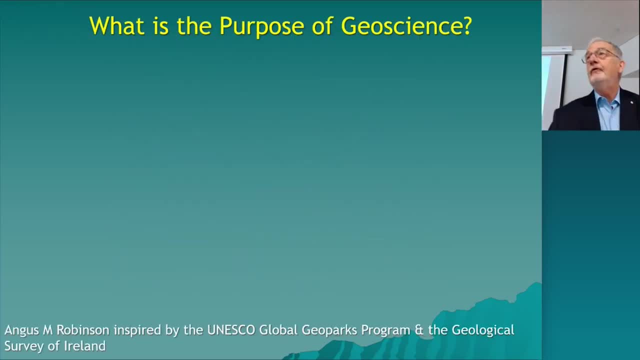 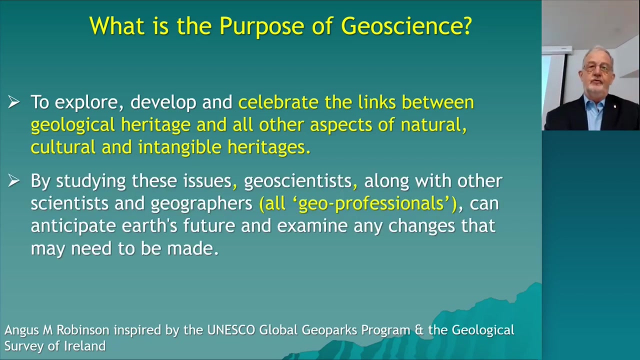 and uh. what i'd like to pose is: what is the purpose of geoscience? now, i think, picking up on what i've read, it's to explore, develop and celebrate the links between geological heritage and all other aspects of natural, cultural and intangible heritages. by studying these issues, geoscientists along with other 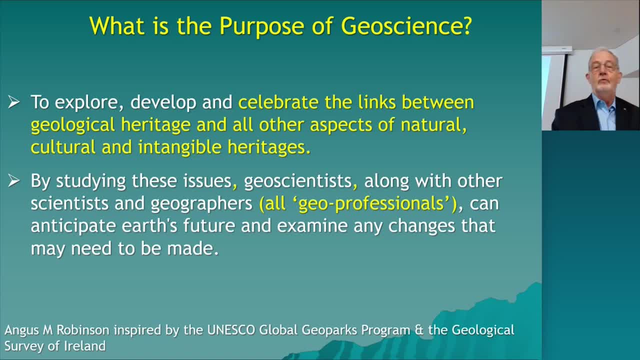 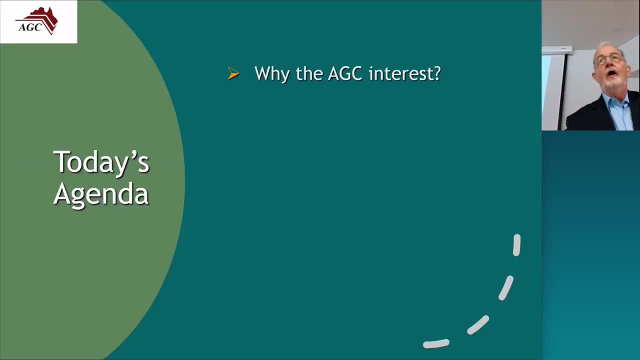 scientists and geographers, or what i would call geoprofessionals, can anticipate earth's future and examine any changes that may need to be made. think about climate change. today's agenda. i want- i want to follow on what rod mentioned about what the agc is about. 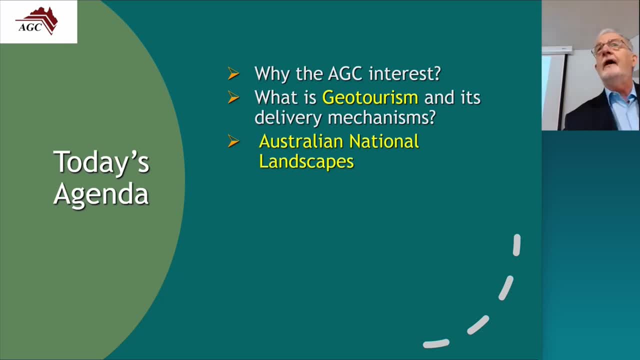 what is geotourism and its delivery mechanisms? a little bit about the australian national landscape program and then to focus on the flinders rangers world heritage area nomination in which geotourism has a important part to play, the national geotourism strategy and then provide 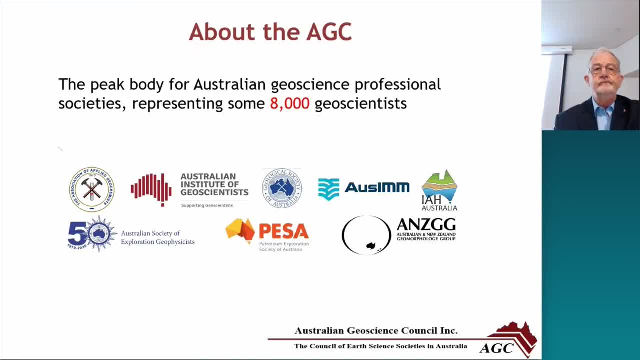 some takeaways now about the agc. it's a peak body for australian geoscience professionals, and each of those professionals have a vested interest in the delivery of the strategy. The AUSIMM and the Geological Society of Australia are the two most active members and have specific roles. 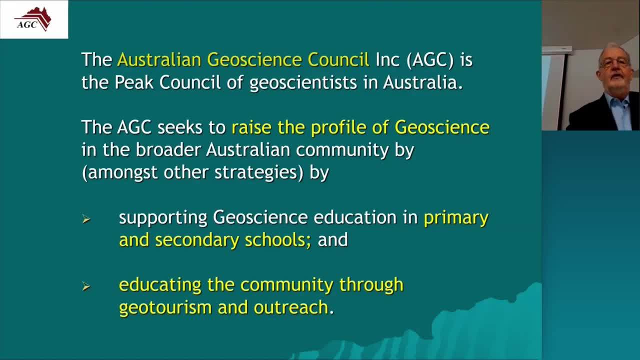 in the delivery of the strategy. Now the AGC as a peak body serves to raise the profile of geoscience in the broader Australian economy and community by, amongst a number of strategies, supporting geoscience education in both primary and secondary schools and educating the community through geotourism and outreach In Australia. we- that is, the AGC- 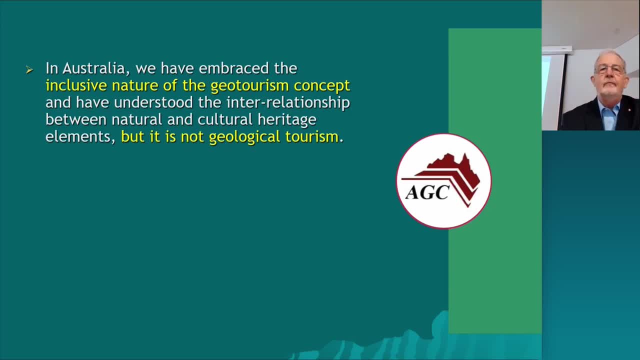 have embraced the inclusive nature of the geotourism concept and have understood the interrelationship between natural and cultural heritage elements. but it's not geological tourism By far. the AUSIMM and the Geological Society of Australia are the two most active members and 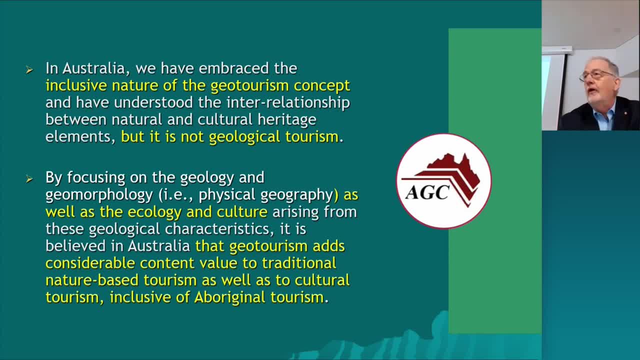 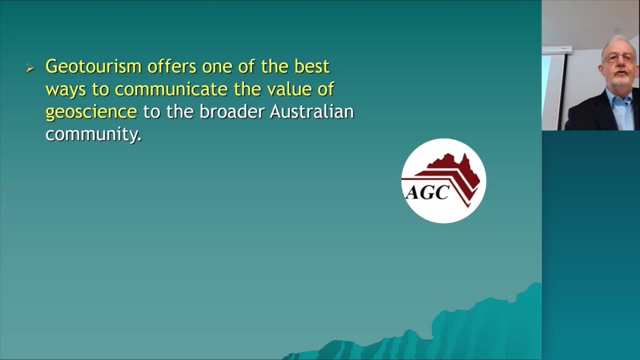 focusing on geology and geomorphology, as well as ecology and culture. it is believed that we can add considerable content value to traditional nature-based tourism, as well as to cultural tourism, inclusive of Aboriginal tourism. We refer to it as enhanced nature-based tourism. in simple terms, Geotourism offers one of the best ways to communicate the value of geoscience. 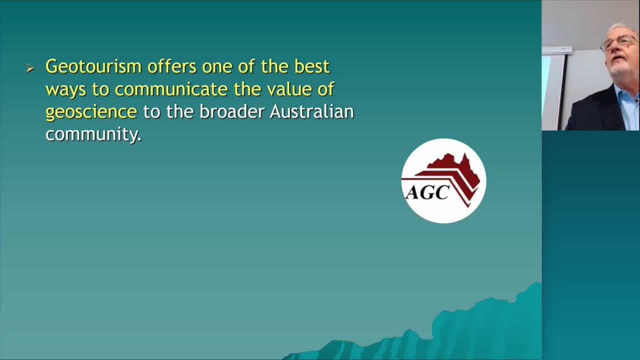 to the broader Australian community. The reason for that is that the AGC is concerned about the drop back of students wishing to pursue earth sciences degrees in Australian universities and, as you all probably know, a number of those universities are closing down courses. Now it is understood from listening what young people are saying. they're looking for a 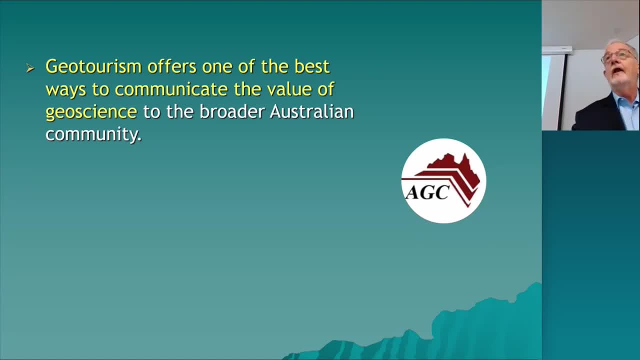 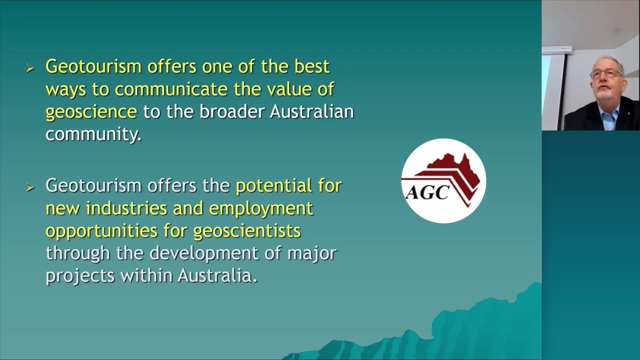 different, more holistic experience across the totality of environmental sciences. So it's important for the AGC to talk to young people, get them out in the field so they can understand what we have to offer. Geotourism also offers the potential for new industries. 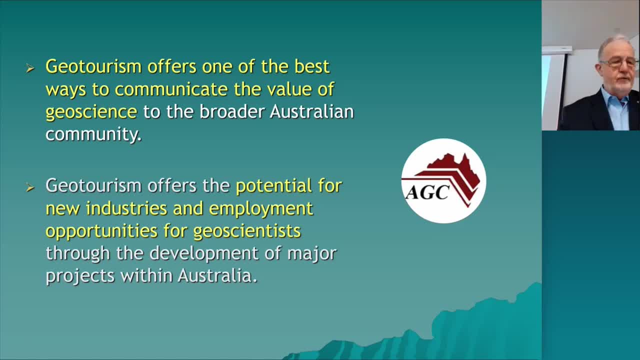 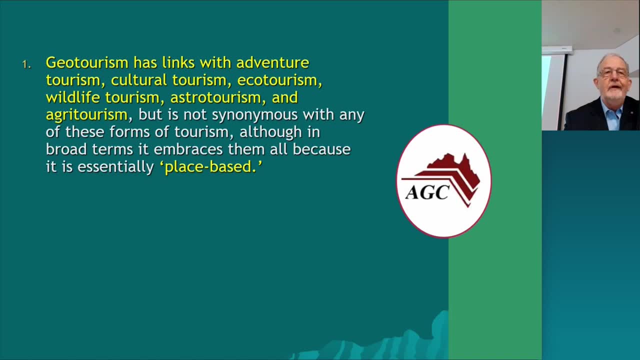 and employment opportunities for geoscientists through the development of major projects within Australia. It has links with adventure tourism, cultural tourism, ecotourism, wildlife tourism, astrotourism and agritourism. It's not synonymous with any of these forms of tourism, although in broad terms it embraces them all. 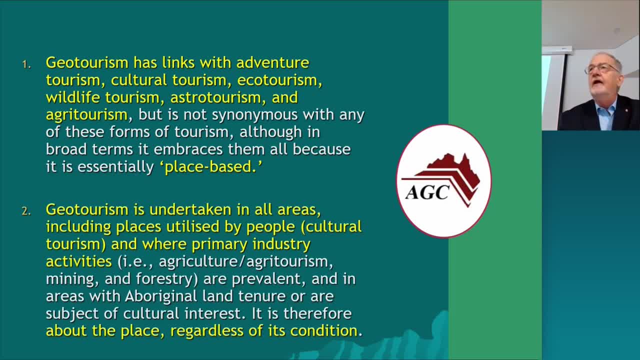 because it is essentially place-based. It's undertaken in all areas, including places utilised by people, cultural tourism, and where primary industry activities like agriculture, mining, agritourism, forestry are prevalent. It is also in areas with Aboriginal land tenure or are subject of cultural interest. The AGC also offers the opportunity for young people to 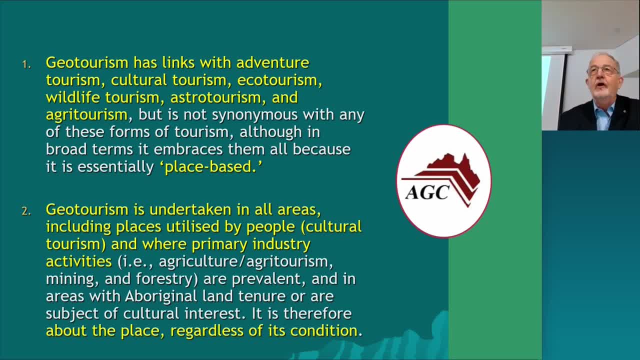 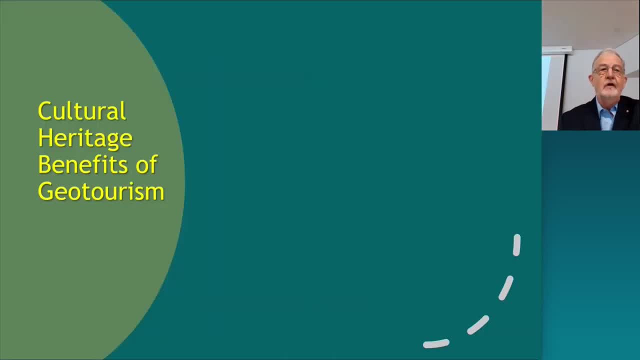 get involved in geotourism. It is therefore about the place, regardless of its condition, irrespective of whether the land is protected or not protected. The cultural heritage of geotourism. we think in terms of holistic Aboriginal culture, in the terms of astrotourism, where traditional 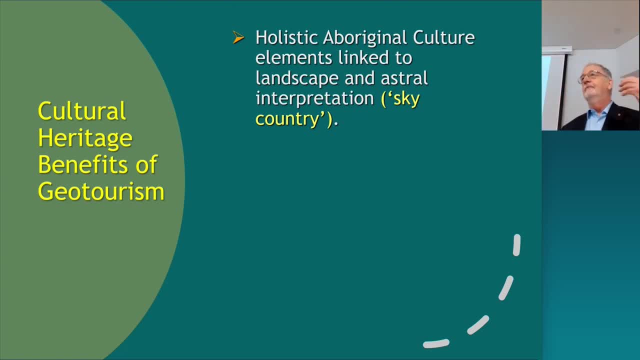 operators are showing people the solar system and things billions of light years away. a level of culturalторы do is how the land is protected, Whereas in fact, as far as the Aboriginal people are concerned, they use the sky to talk about how it relates to their landscape. So we're 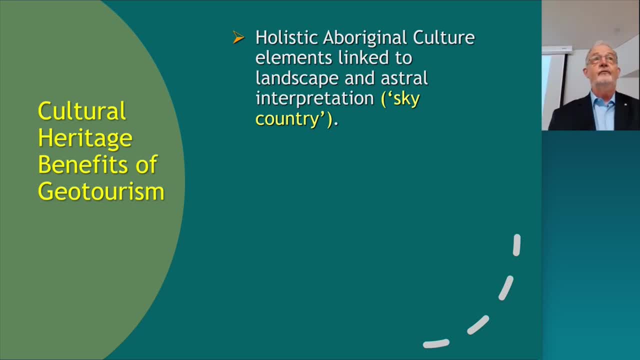 putting the idea in people's mind. that's what's really going to be important about the place, because each place around Australia has a different experience because of the Aboriginal cultural aspects. For an Australia, enhanced understanding of cultural elements or a whole range of post-European settlements, extensive mining heritage and other cultural heritage-based areas. we can design an overall approach to geotourism with more cultural heritage. If someone has been interested in the setting of geotourism, it is meant to be an approach to learning the world's cultural heritage. 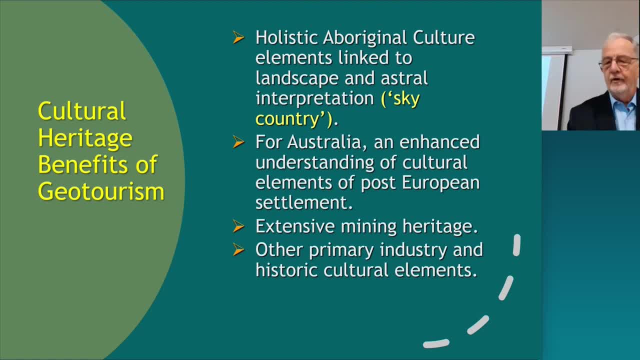 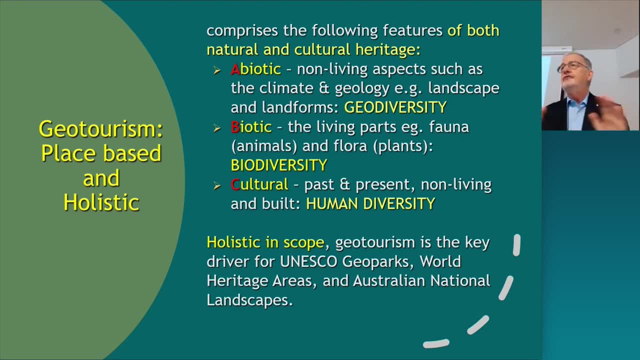 The interests of the Australia-based gli, the need for social dialogue, the need for cultural and other primary industries and historic cultural elements. They are all important and part of the mix. Now, essentially, to try and simplify this, we say geotourism, place-based and holistic. 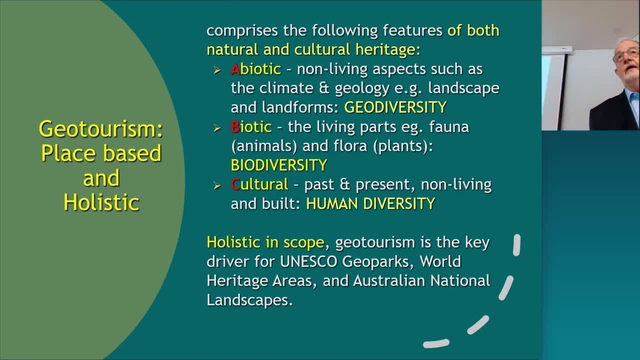 encompasses three elements: the A, the B and the C. A is biotic, which is geology, landscape, climate, et cetera. Biotic is flora and fauna and C is culture, both Aboriginal and post-European settlement. 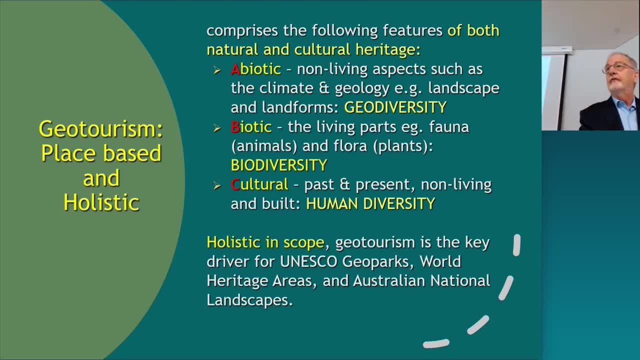 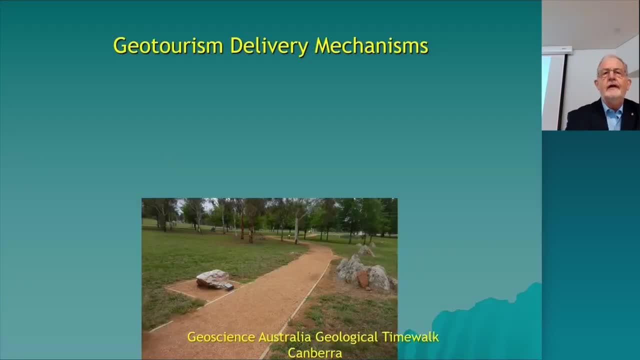 So we talk in terms of identifying the A plus B plus C characteristic of every potential geotourism experience. Now there are various delivery mechanisms for geotourism. First of all, there's geosites and mining heritage sites. That's just where rocks outcrop or where mines are being built. 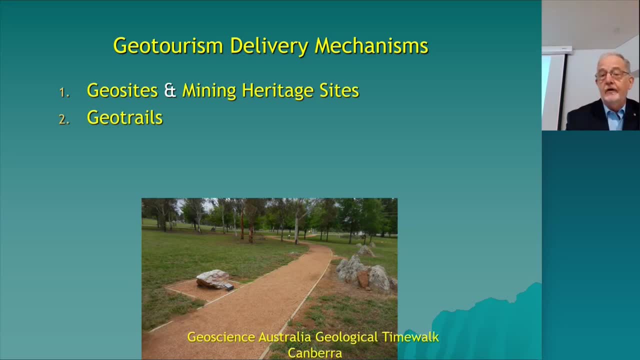 Secondly, geotrails, which are journeys between sites, and I'll say a little bit, a little bit more later in the presentation, geoparks and world heritage areas, and I'll speak briefly about those, And, of course, geological time walks and rock gardens. 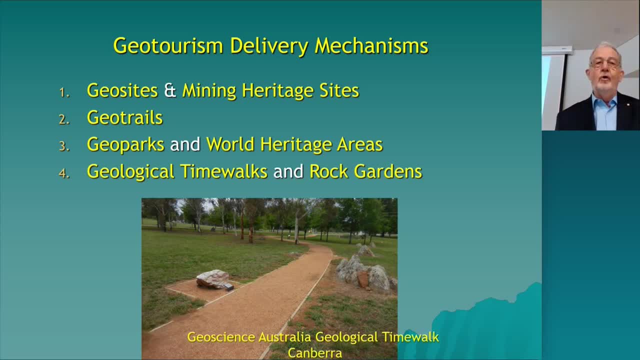 Well, here in Canberra we have a 1.2 kilometre time walk which outlines the course of geological history in Australia, And it's the best example we have in Australia and I recommend a visit to it. But we also have the National Rock Garden. 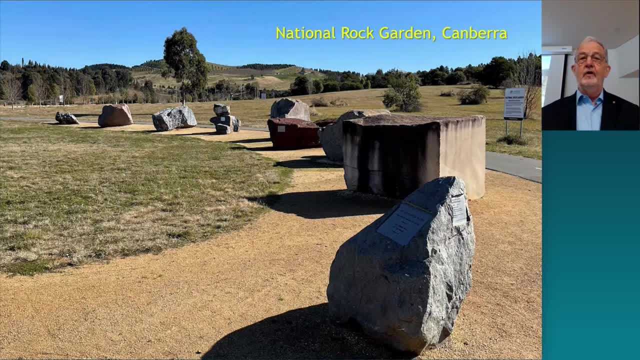 which has now been built, and it's located next to the Arboretum, which puts in place specific exemplars of rocks that have been transported from anywhere around Australia, particularly by donors and mining companies, And that in itself tells the story. These are mechanisms based on geology. 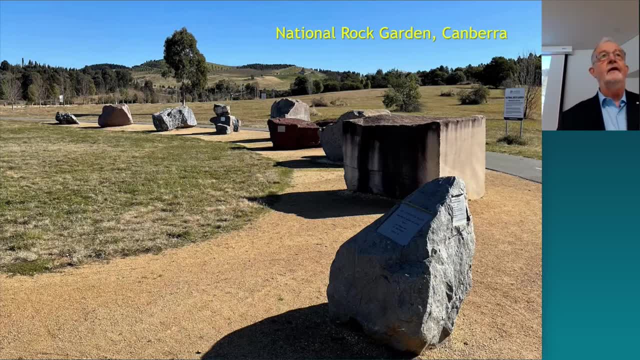 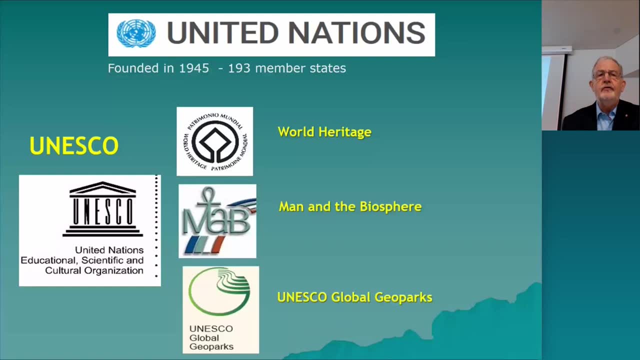 but don't pretend to have aspirations of incorporating biotic or cultural elements. Cultural, perhaps because it's important to geologists. Now, in terms of the the United Nations programs, there are three areas of activity: world heritage areas, Man in the Biosphere and UNESCO global geoparks. 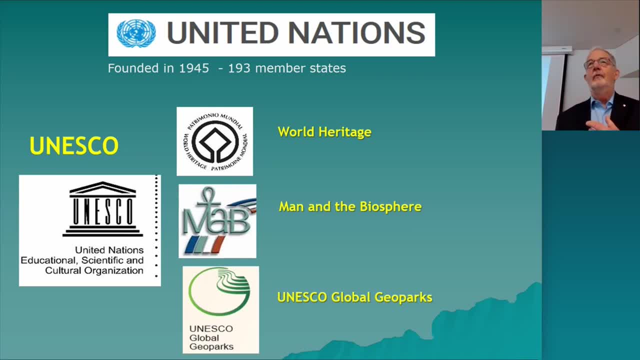 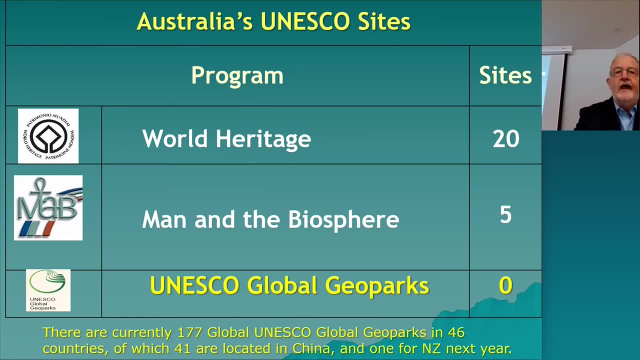 all representing different ways in which people relate to the environment, across both natural and cultural heritage. In Australia, when we look at the UNESCO sites, we have 20 world heritage areas. You'd be familiar with: the Barrier Reef, Blue Mountains, Stone Tree. 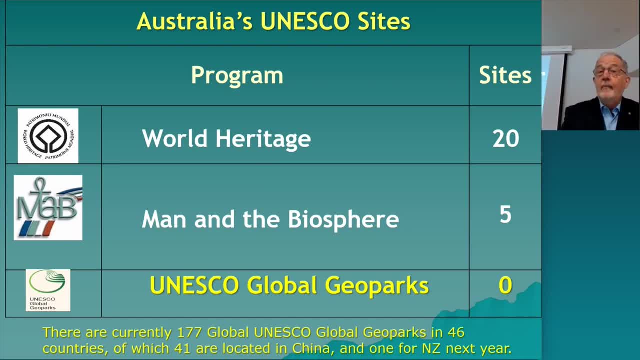 Lamington National Park and so on and so forth. We have five Man in the Biosphere areas- The last one was declared last June- and zero UNESCO global geoparks, And that in itself is a is causes some concern, because there are 177 UNESCO global geoparks in 46 countries. 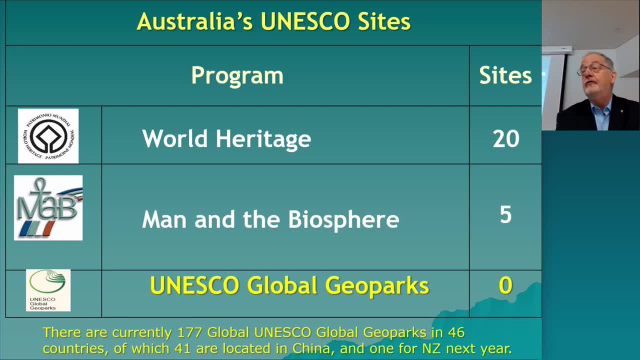 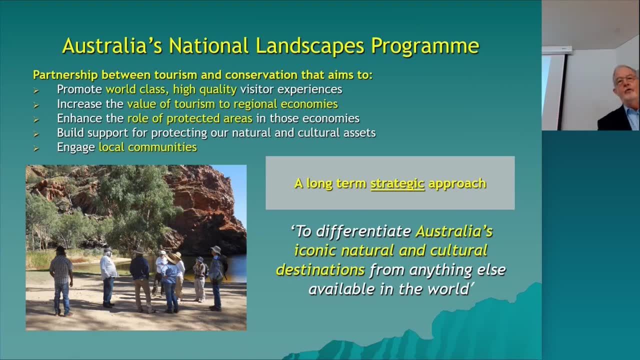 of which 41 are located in China and one for New Zealand next year, And we want to try and do something about that. But we did have a program called the Australia's National Landscape Program, started in 2005, supported by Tourism Australia and Parks Australia and attempted to be able to create a partnership. 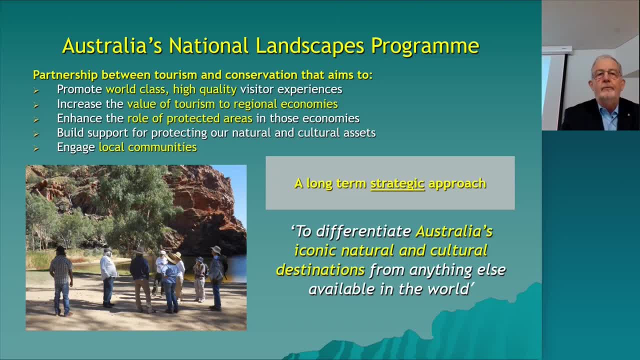 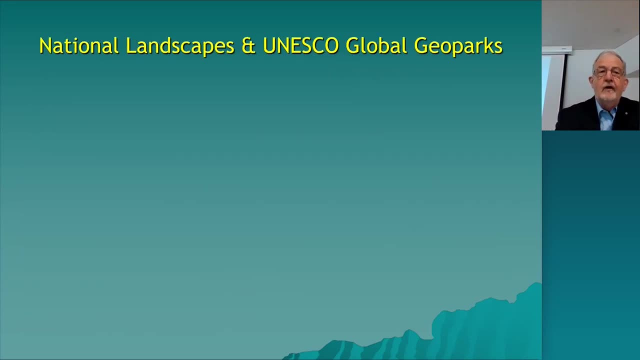 which promoted high quality visitor experiences, looked at protected areas, engaged with local communities. It was a long term strategic approach to differentiate Australia's iconic natural and cultural destinations from anywhere else in the world. But unfortunately that program, whilst it did have similarities with UNESCO global geopark program as it related to community engagement, 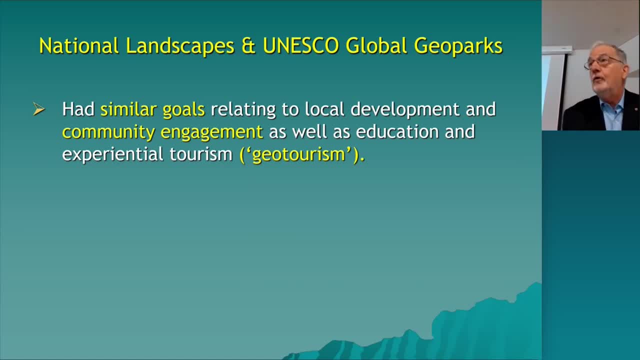 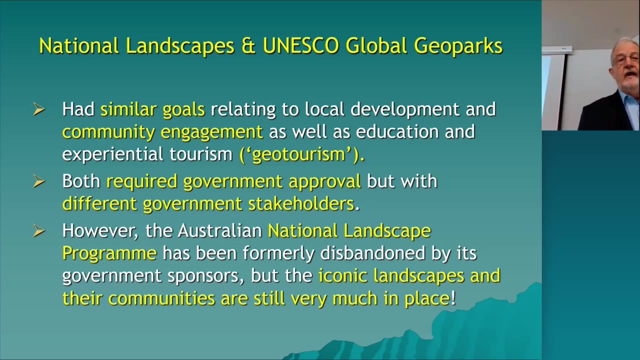 education and experiential tourism- we call that another word for geotourism- And whilst they both require government approval, but with different government stakeholders, unfortunately, the program was disbanded in 2014 for various reasons, And we make the point. 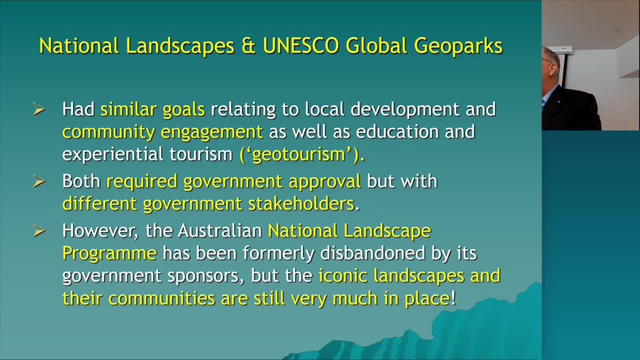 although the program was disbanded in 2014,, the program has has been dispensed with. the landscapes are still there, The communities are still there and there are an opportunity to look at those landscapes and see which way that they can be developed for geotourism purposes. 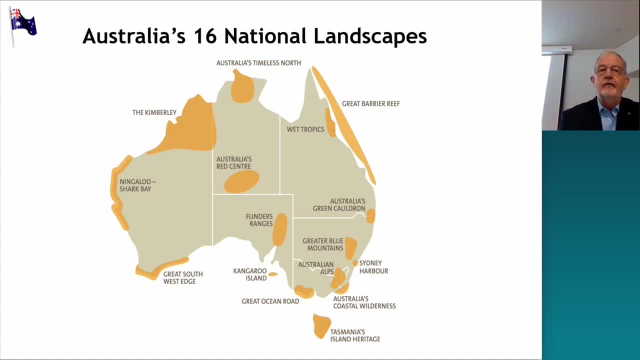 Those 16 national landscapes are listed on this map, and the areas would all be familiar with you, I'm sure, But I want to focus on one of those areas, which is the Flinders Ranges. The Flinders Ranges is an important area. 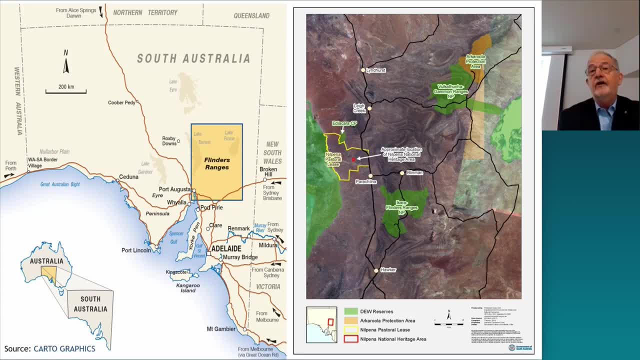 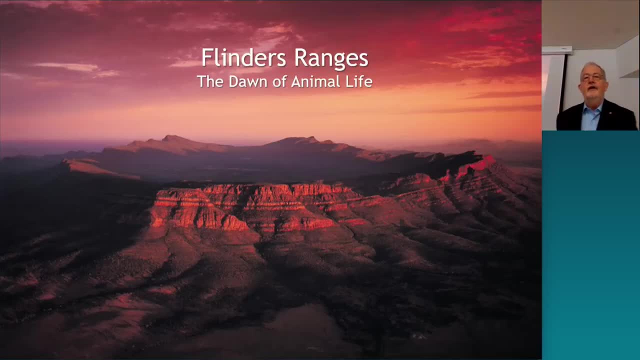 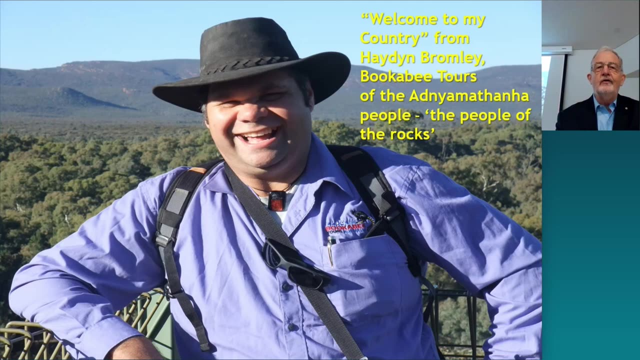 And, but it's significantly a subject to a World Heritage nomination at a very advanced stage. It's been positioned as the dawn of animal life, And the reason for that I'll explain in a moment. but I also would like to convey a welcome from my good colleague. 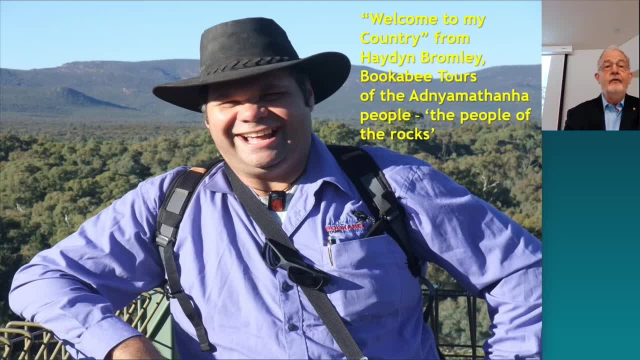 Hayden Bromley of Booker B Tours. He's of the admin for people in there. That's a word for the people of the Rocks. now we're very fortunate to have Hayden on board as a member of the National Geotourism Strategy Steering Committee. 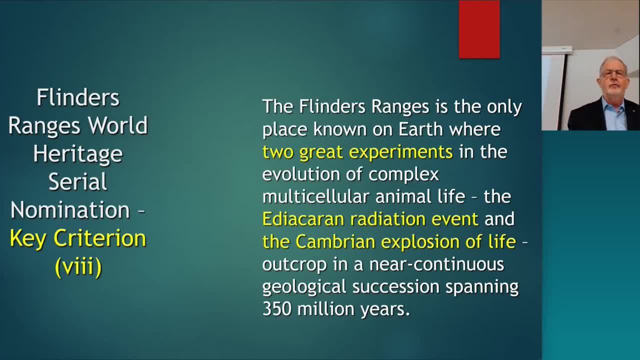 And he's a great contributor. Now the Flinders Ranges World Heritage Serial nomination in the criteria, criteria number eight, states that the Flinders Ranges is the only place known on Earth with two great experiments in the evolution of complex multicellular life. The 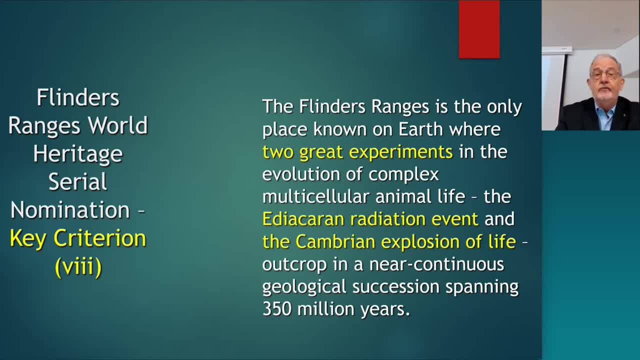 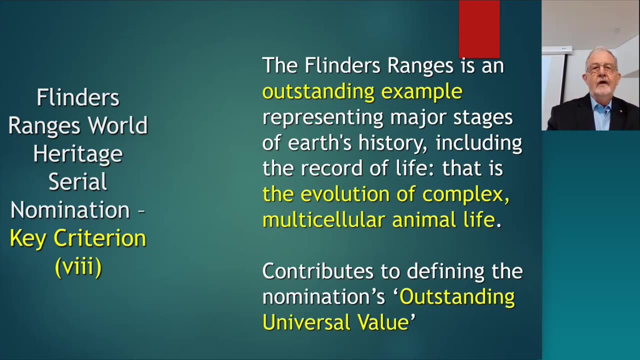 And Ediacaran radiation event and the Cambrian explosion. life outcrop in a near continuous geological success in spanning 350 million years. That's the key criteria. The Flinders Ranges is an example representing the major stages of Earth's history, including the record of life. 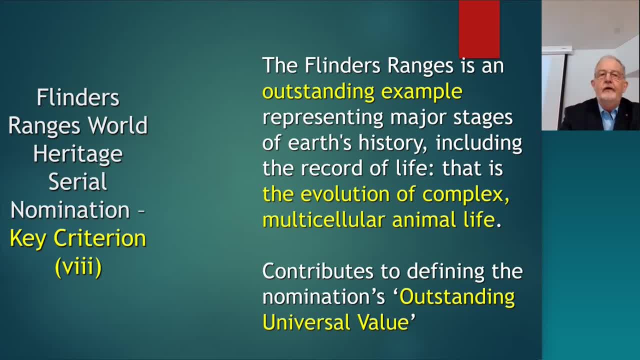 As I've said, that is, the evolution of complex multicellular life. The Flinders Ranges World Heritage Serial nomination in the criteria, criteria number eight states that the Flinders Ranges World Heritage Serial nomination in the evolution of complex multicellular life. 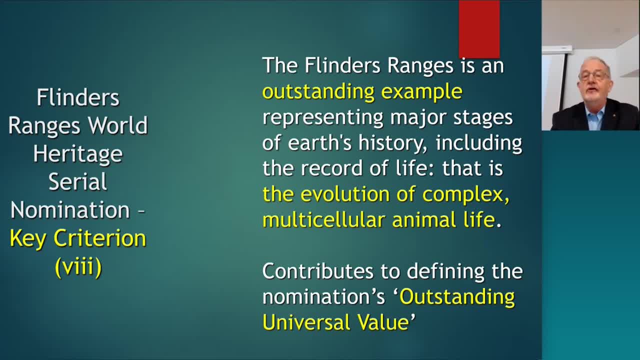 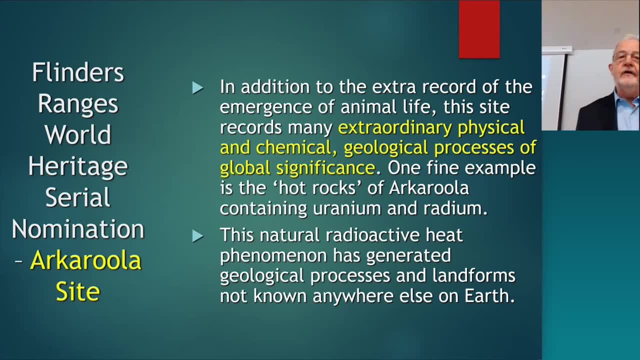 and that's explained by the definition of multicellular life as the ultimate goal of modern human and conserved animal life. It contributes to defining the nominations outstanding universal value. Also, it incorporates the Arcarula site in the northern part of the Flinders Ranges. 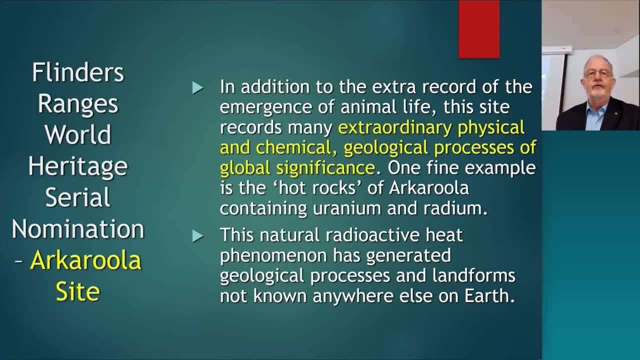 where demonstrates extraordinary physical and chemical processes of global significance, which is related to the way the geology has been transformed over the years, so to speak, And it's a process that's not simple, simply seen anywhere else in the world. The geotourism potential is there. 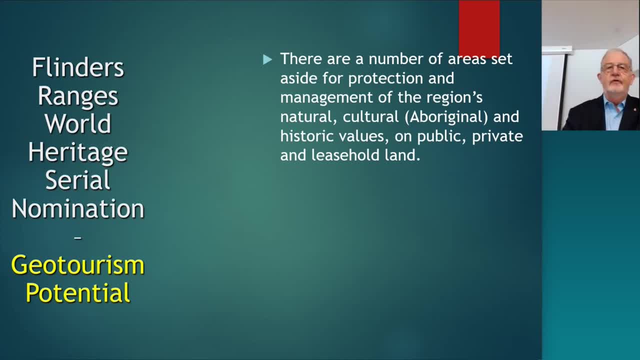 We think there are a number of areas that can be set aside for protection and management of the region's heritage on both protected, private and leasehold land. Pastoralism has had a strong historic influence in the region and continues to be an important industry today. 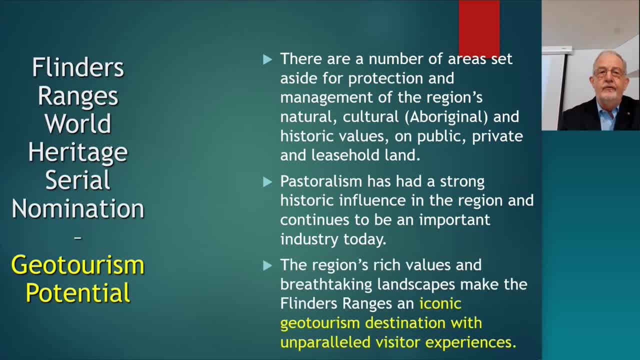 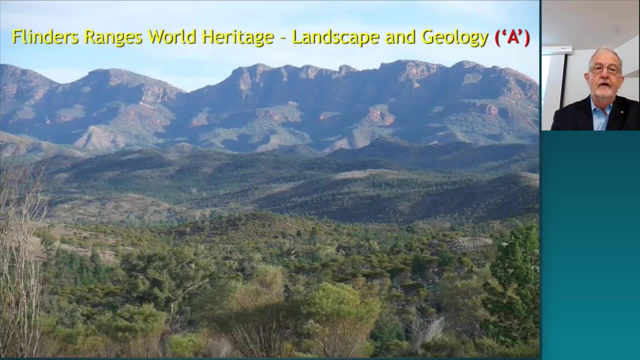 and there are active communities wishing to be involved in this process. The rich values and breathtaking landscapes make the Flinders Ranges, we believe, an iconic geotourism destination with unparalleled visitor experiences. Now let's look at the A plus B plus C. 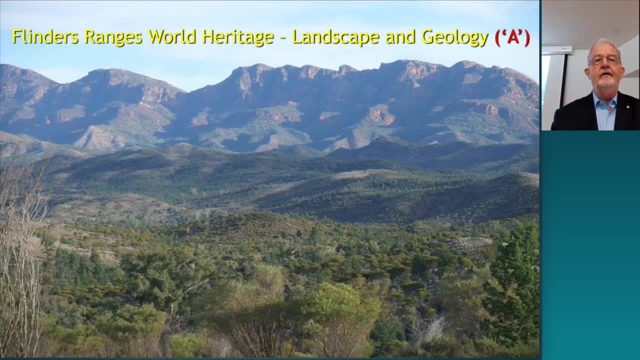 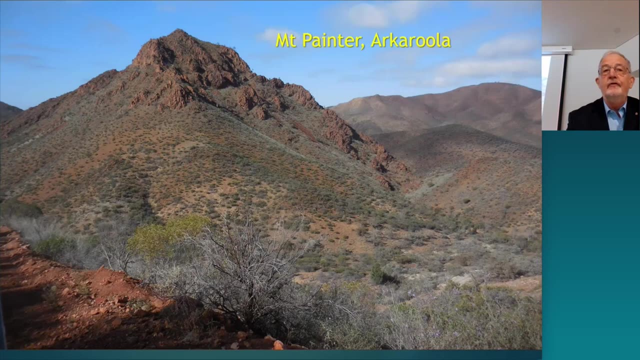 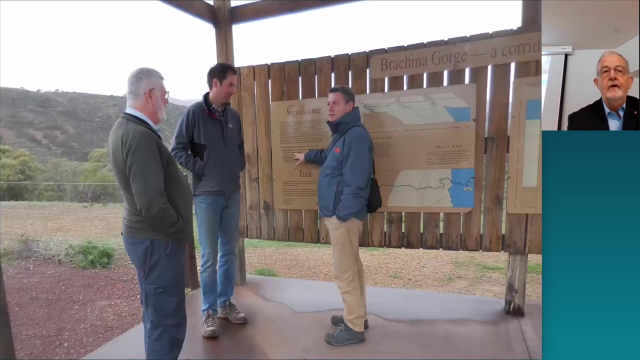 There we have the Wilpena Pound and it's a very beautiful landscape. We have the Karula landscape. quite different, rugged Mount Painter is a very well known landform in that area. We have the work that's been done in the 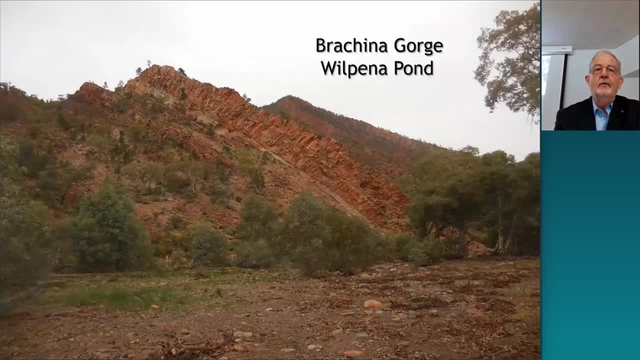 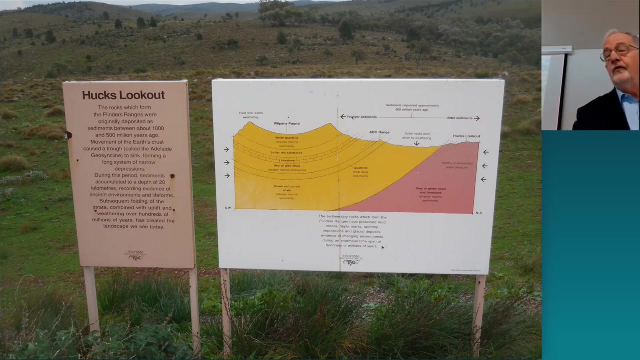 development of the Brackina Gorge Geotrail. There we have the geology there quite straightforward, and what the Geological Society of South Australia have been able to do is to put in place signage which actually helps explain the geology along the course of that particular geotrail. 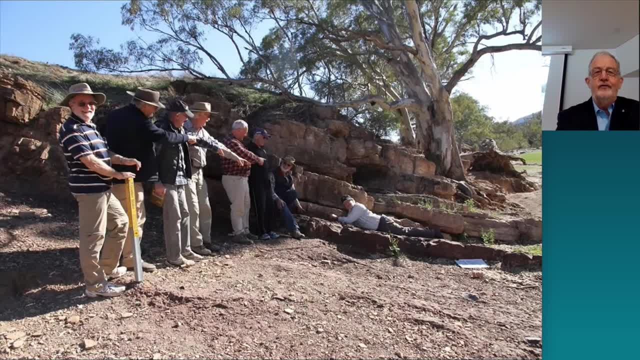 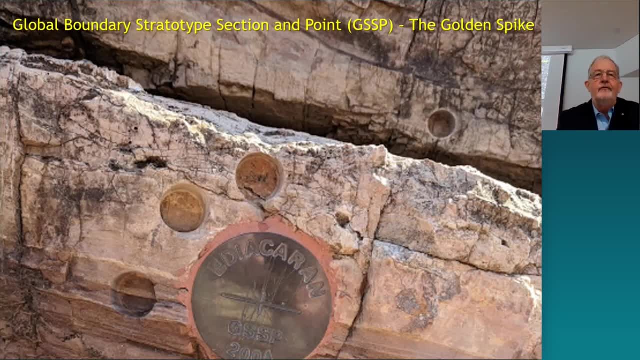 But it's a very important point. There's our geologists getting quite excited about a particular location. That location is the Global Boundary Stratotype section and point for the GSSP, in short terms called the Golden Spike, and identifies the basal segment of the Ediacarum strata. 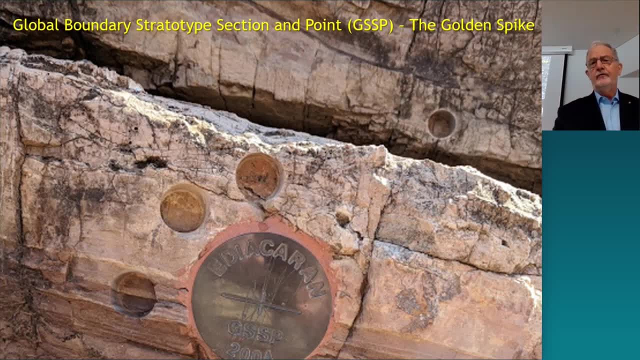 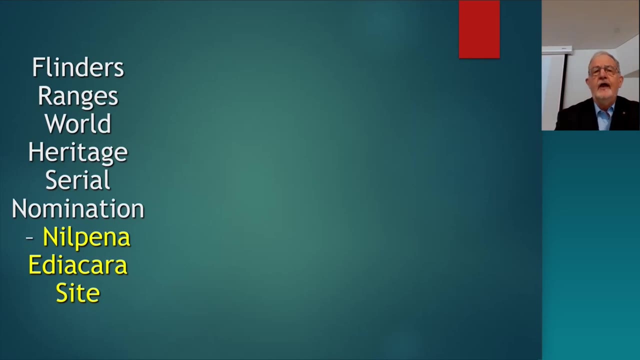 Very important, and the National Parks are doing a lot of work to be able to make that that site both safe from vandalism but also accessible for visitors. Now, when we look at where the Ediacarum fossils have been located, there is what's called the 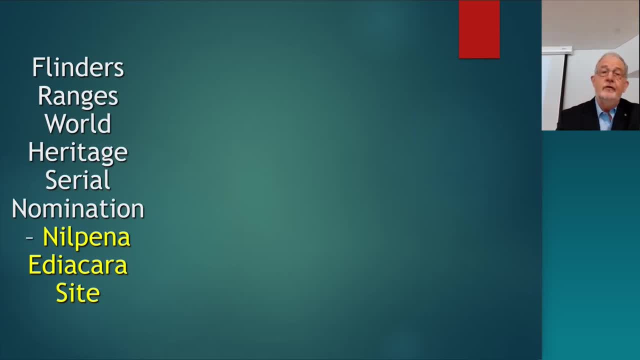 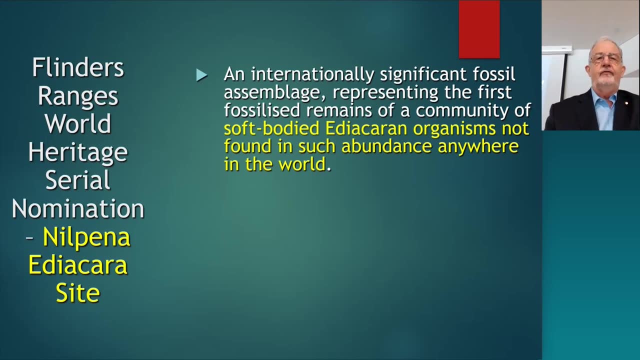 Nilpena Ediacara site, now part of a new national park within the World Heritage Nomination Area. It is an internationally significant site because it shows the fossilised remains of a community of soft-spreaded Ediacarum, organisms not found in such abundance and variety. 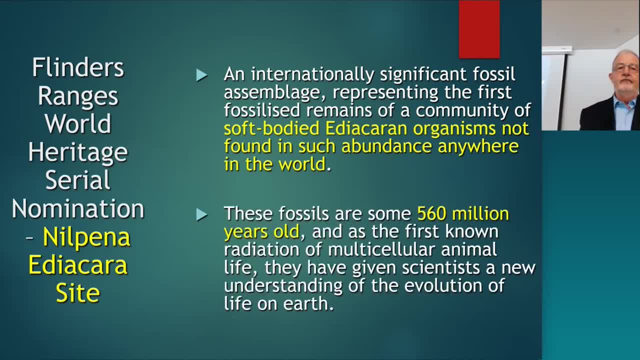 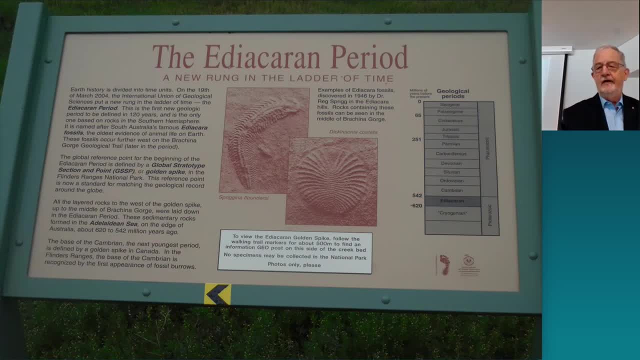 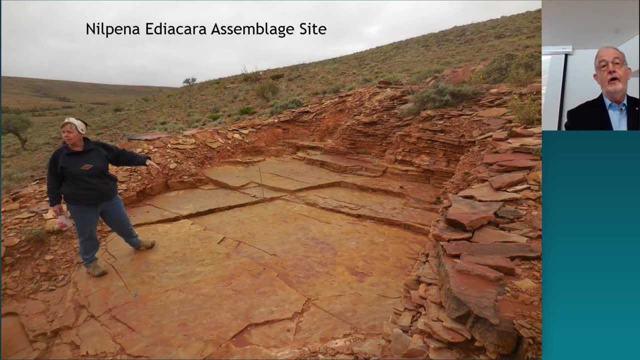 anywhere else in the world. These fossils are some 560 million years old And there's information there about them, well explained. in the World Nomination Area There's the site itself. Professor Mary Droser has done a lot of work in the identification of those fossils. 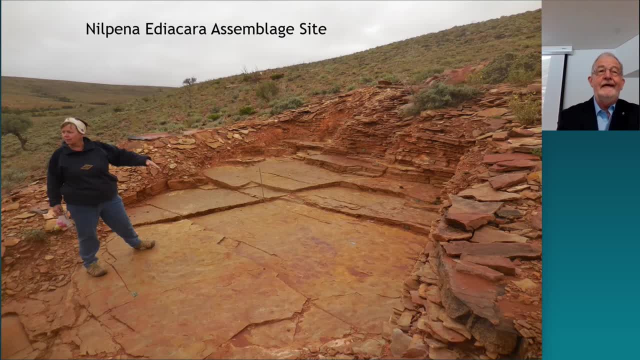 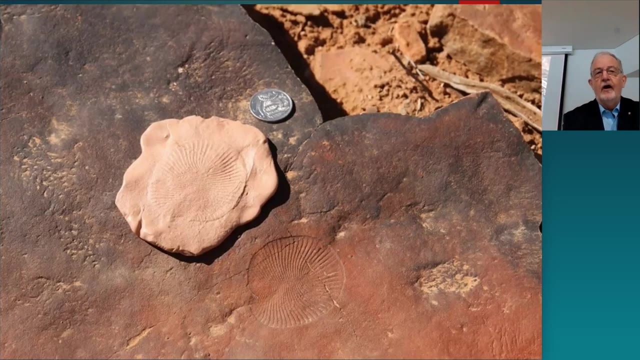 over quite a few years And that's known as the Nilpena Ediacara assemblage site being protected and will may be made available for visitations very shortly. The fossils there are small. Give you an idea the size of them. 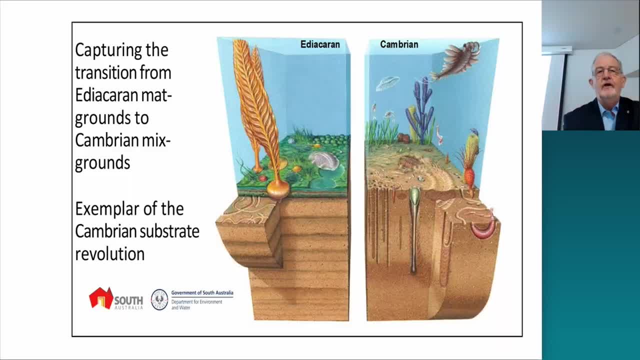 they're small but they're quite, quite interesting in the way that they have developed. And when you look at the, how does that compare to the fossils that we're more familiar with in the Cambrian assemblage? on the left hand side you have the these: 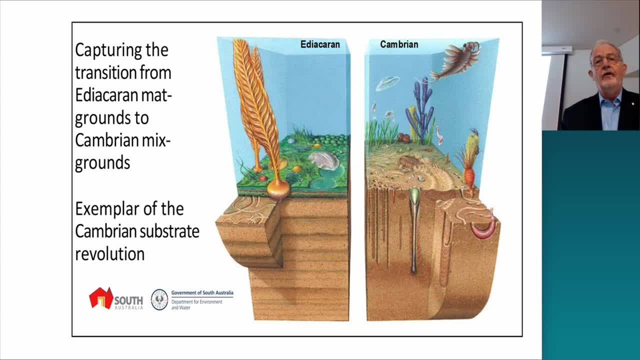 wavering single cellular organisms And on the right hand side, the Cambrian assemblage of trilobites and other fossils. other species have been developed, So that's basically the story of the fossil assemblages in the World Heritage Nomination site. 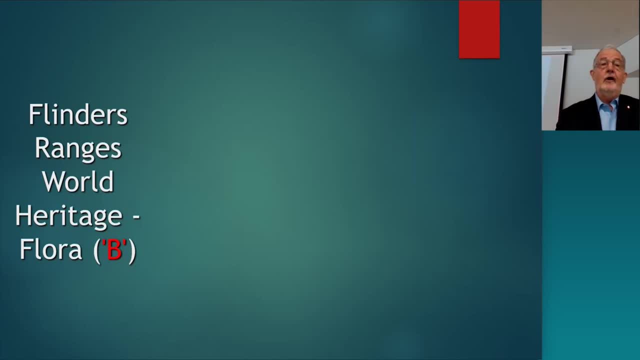 Now let's look at the flora of the bee, the biotic elements of the Flinders Ranges World Heritage Area. There's a whole range of of fossils of sorry plants that are dependent on on the conditions relating to geology. 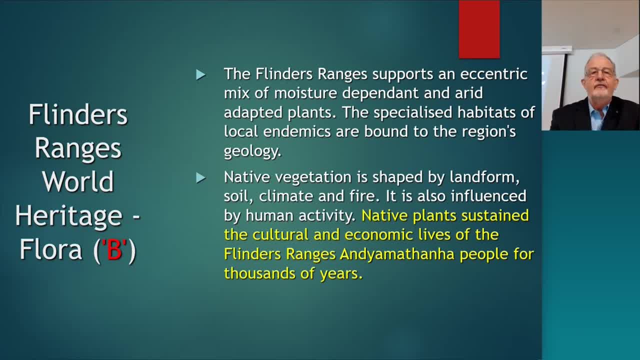 It's also influenced by human activity. Native plants sustain the cultural and economic life of the Flinders Ranges and demand for people for thousands of years, And that's the story in itself. And there's at least 85 plant species in the Flinders. 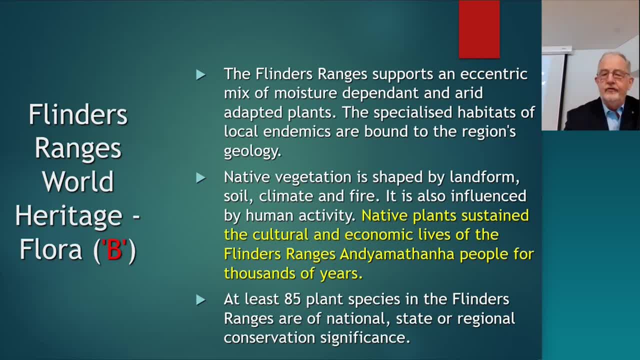 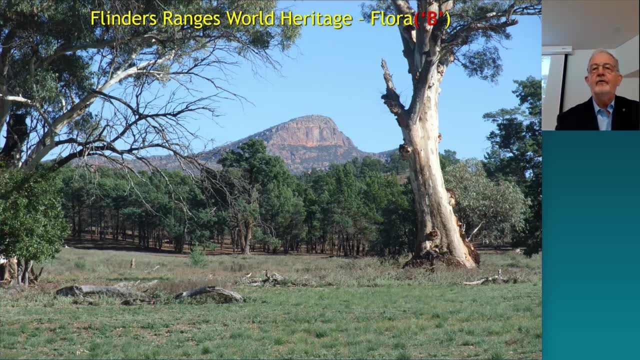 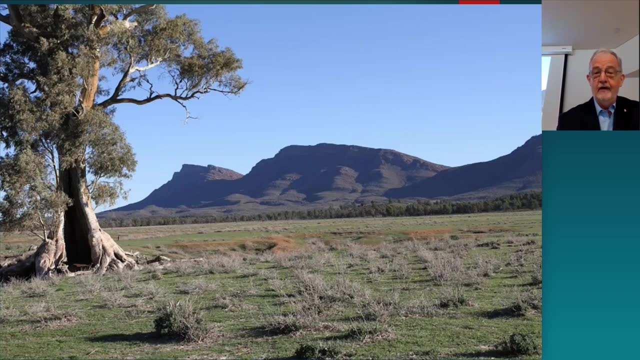 Ranges are of national, state or regional conservation significance. We look at the kind of flora we have there. this is very typical of the looking across the Cyprus Pined the famous canyons for a red gum tree. That's well visited, famous landmark. 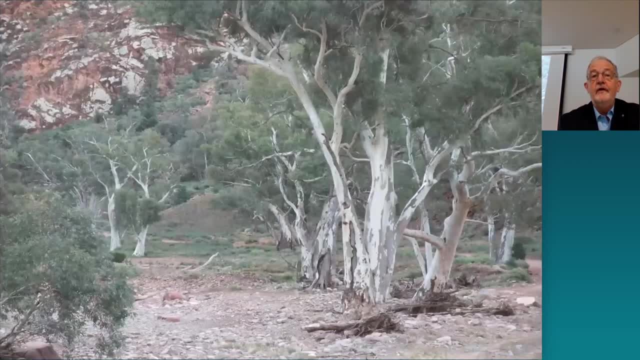 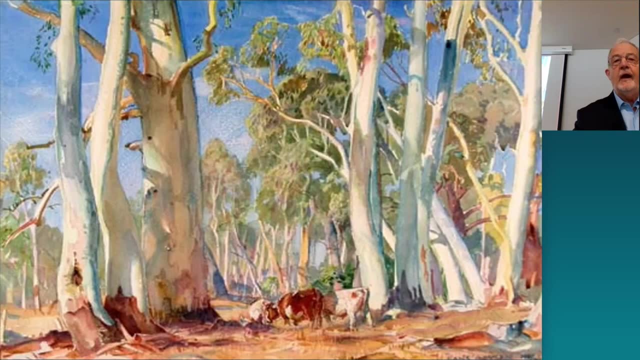 again more vegetation, and then the red gums. The interesting thing about the red gums: it's quite spectacular across central Australia and northern ranges and it's been captured by the paintings of Hans Heysen. So if you're going to the Adelaide, 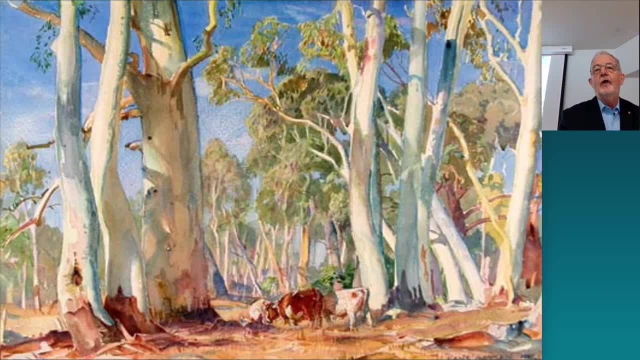 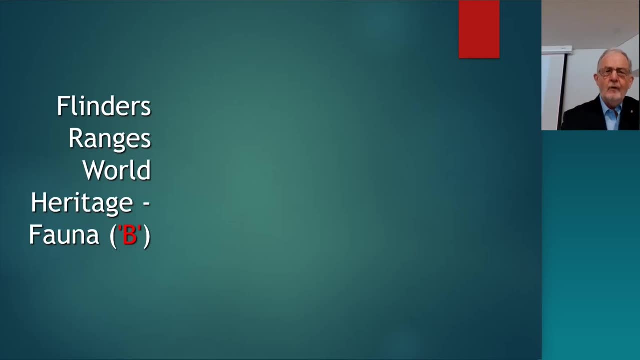 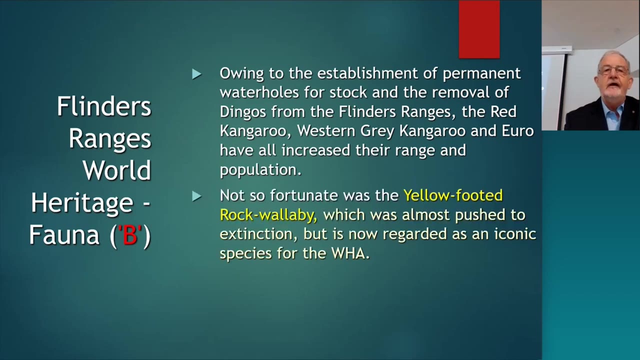 I do recommend a visit to the Art Gallery, and the paintings will all come to life after you've been to the Flinders Ranges. They're beautiful paintings. When we look at the fauna, plenty of kangaroos, euros have increased their range and population over the years. 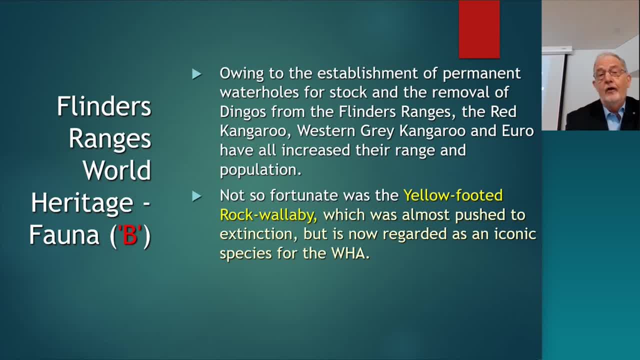 And, but not so fortunate, has been the yellow footed rock wallaby, which was almost pushed to the extinction, but it's now regarded as an iconic species for the World Heritage Area. It's also a very important species as far as the Aboriginal people are concerned. 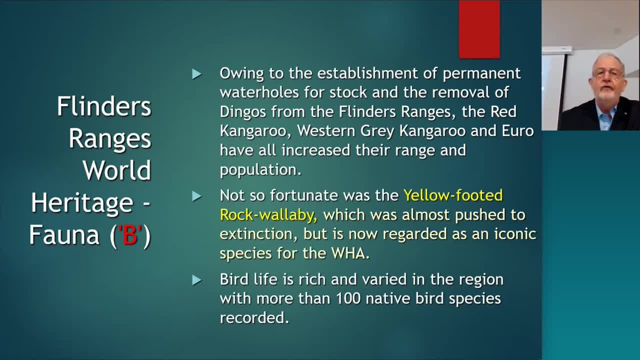 Bird life is rich and varied in the region, with more than 100 native bird species recorded. That's important because we find a lot of geologists love bird watching. It's an activity which appeals to geologists If you go through the Flinders Ranges. 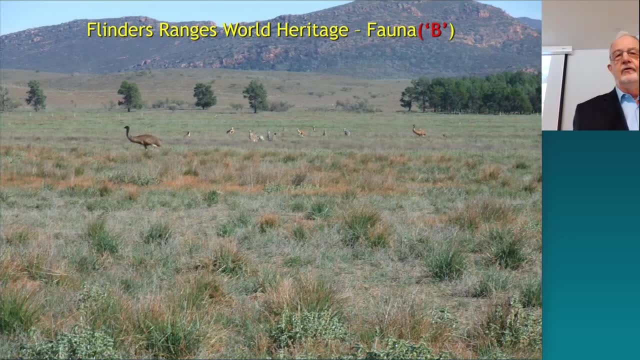 there's wildlife, plenty to see- kangaroos, euros, emus- And I might say that's not the story. you know, you see a lot of other places in Australia where you see such a rich abundance of native wildlife. Yeah, 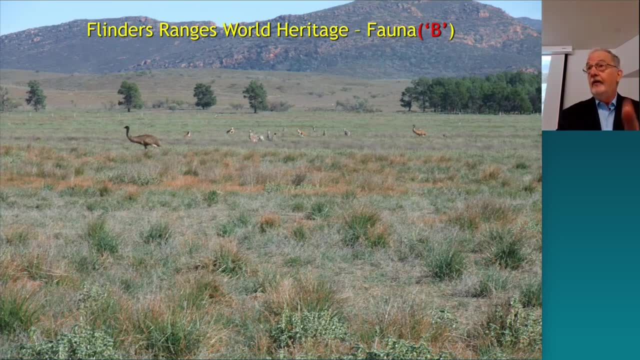 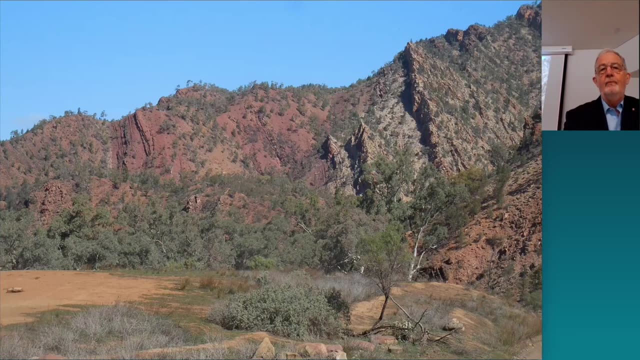 we see kangaroos and the occasional dead dingo, but here in the Flinders Ranges it is rich in wildlife. The actual geology provides wonderful habitats for the yellow footed wallaby. the scree slopes along those hills. Now you can see the yellow footed wallaby is well disguised. 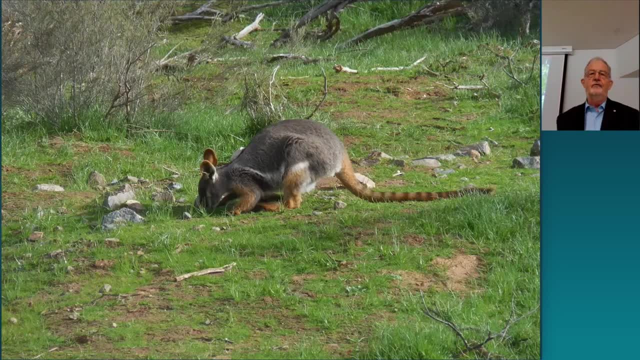 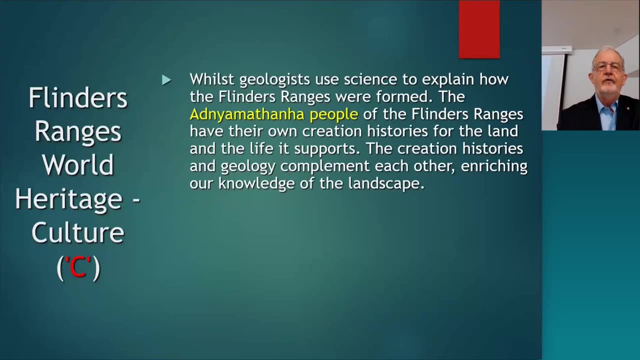 but you can see the yellow footed wallaby is well disguised in that particular environment. When it comes out into grass you see what a beautiful animal he is. The culture is also important- The people. there's a great relationship between the Aboriginal people. 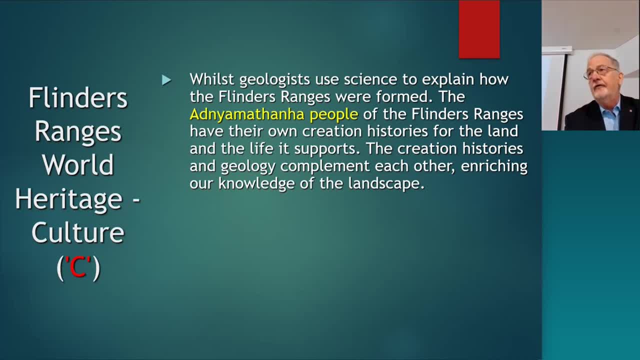 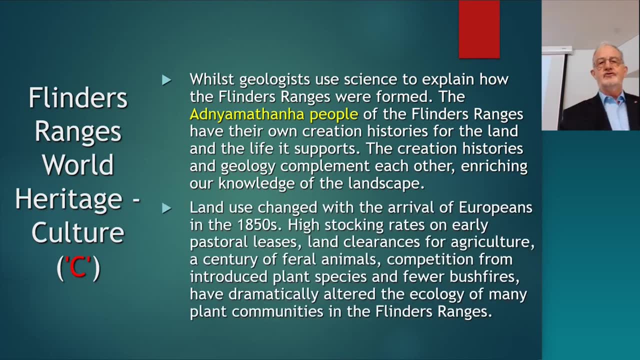 the way that they have interpreted the environment and how they can relate landscape to astrotourism, as I mentioned previously, And there's a lot of land use that has changed the way in which Europeans have operated, and I think that's quite interesting. 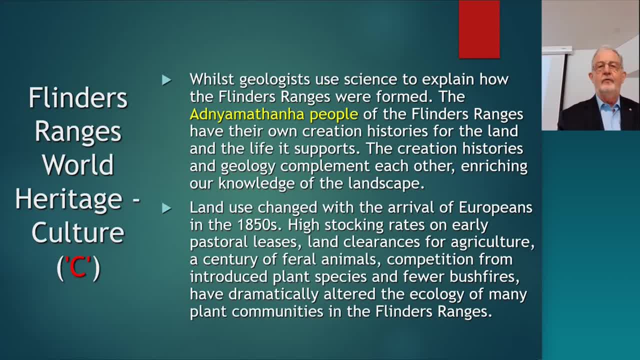 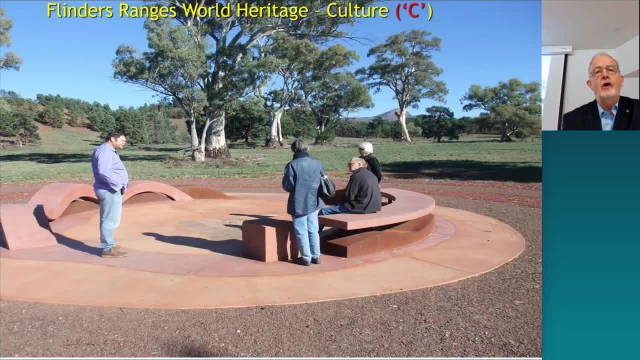 I think that's quite interesting, The way the area has been cleared and fenced and, one thing or another, the impact that's had on the ecology of the area As far as the Aboriginal culture is concerned, in the Ikara National Park in Wilpena Pound. 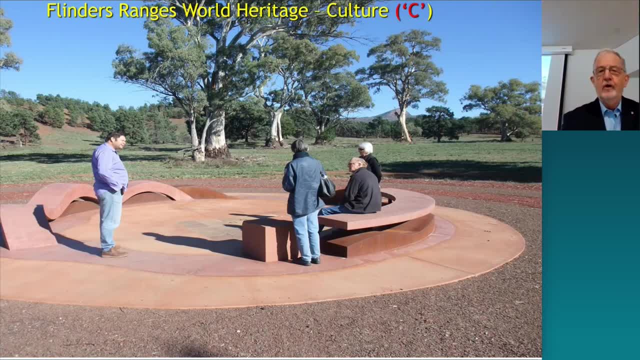 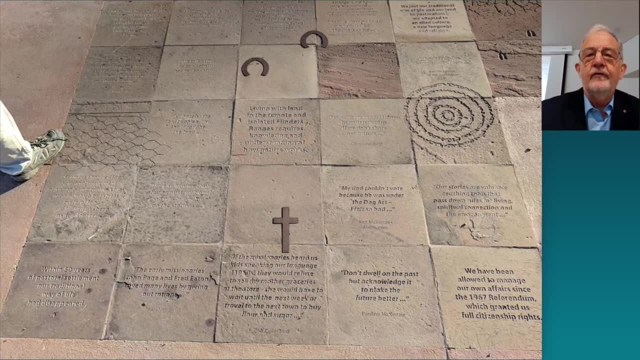 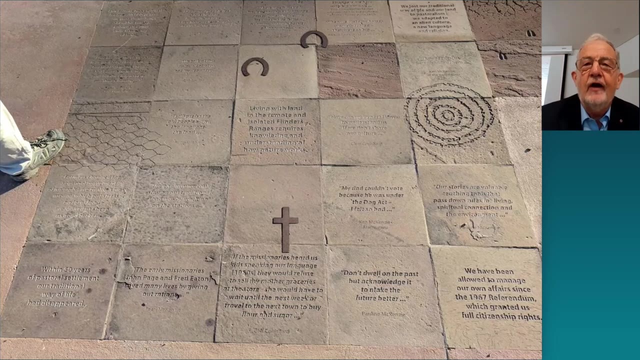 they have a particular, let me say, exhibit which explains various stories that Aboriginal people have had. There's one there it says our stories are with the, with these whatever passed down ideas in living, spiritual connection and the environment. So there's various perspectives that are set out in these series of exhibits. 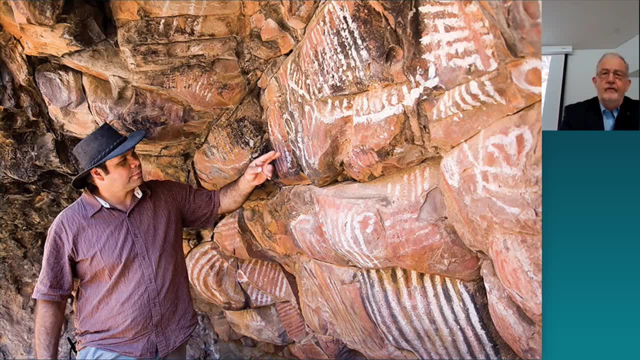 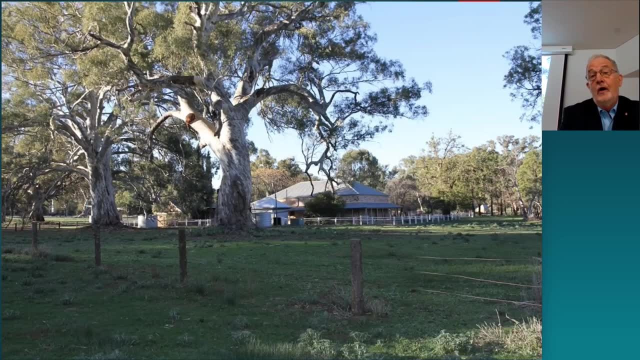 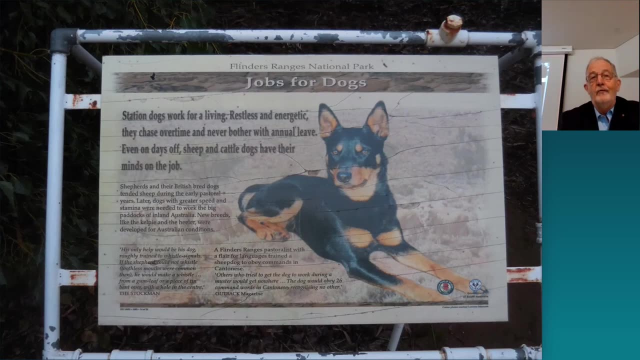 And of course there is the art work as well, rich in the Flinders Ranges. Moving on to European culture, you've got the Wilpena old homestead there and its pastoral history. They also celebrate the work of the cattle, dog or sheepdogs over the years. 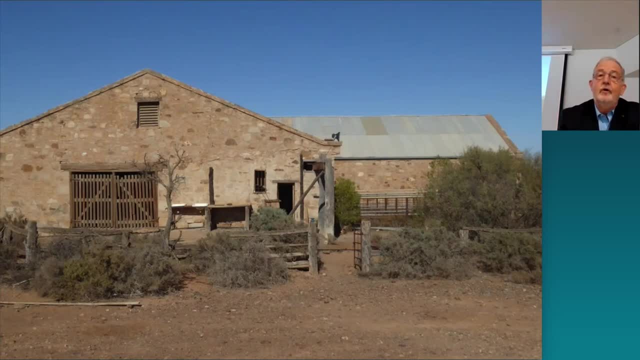 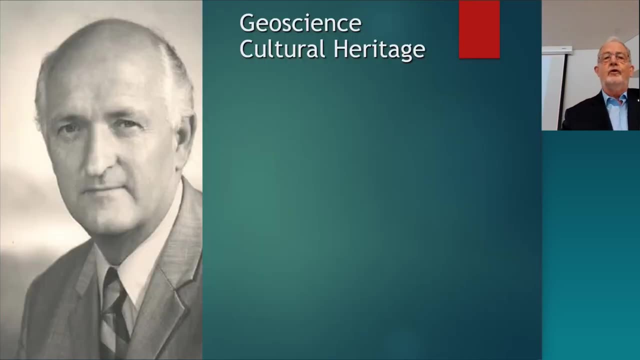 celebrate some of the original architecture of the original buildings. That's all part of the cultural heritage. There is another part of cultural heritage that we think is very important and that's the work of the original geologist, Dr Reg Spriggs, who was mentored by his friends. 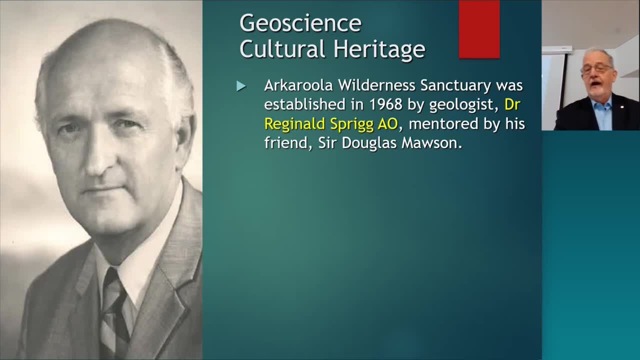 Sir Douglas Mawson, who in fact discovered the Ediacaran assemblage quite some years ago. But significantly, Dr Spriggs has created a conservation area in Arkabrulla and set aside for the protection of the environment, And his family have been able to maintain that and develop that as a world-class. 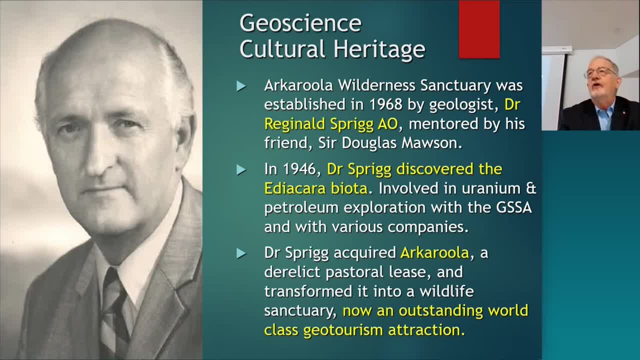 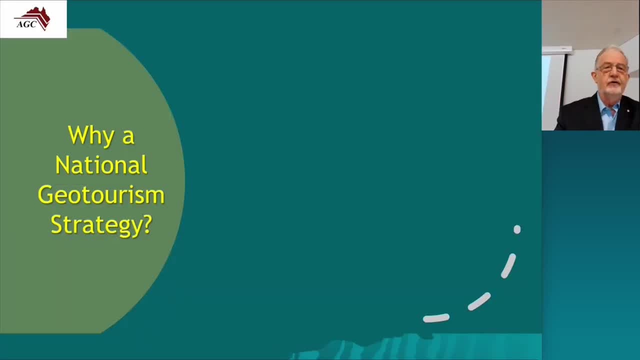 outstanding geotourism attraction. He's very much part of the geoscience culture of this country. Now let's look at the whole issue of a national geotourism strategy. Why do we need a national geotourism strategy? 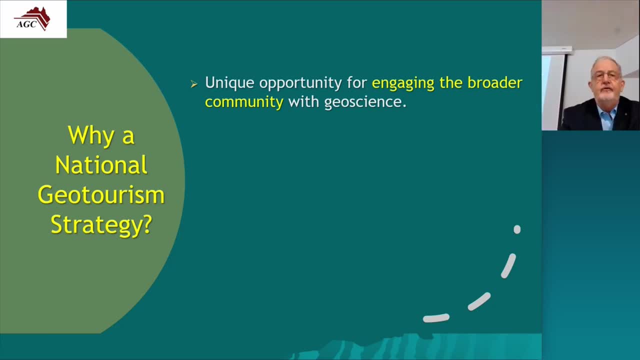 As I've mentioned, it's an opportunity for engaging the broader community with geoscience, With COVID. domestic tourism needs to be able to find new ways of building product development, to bring tourism to look at our own country rather than just traveling overseas. 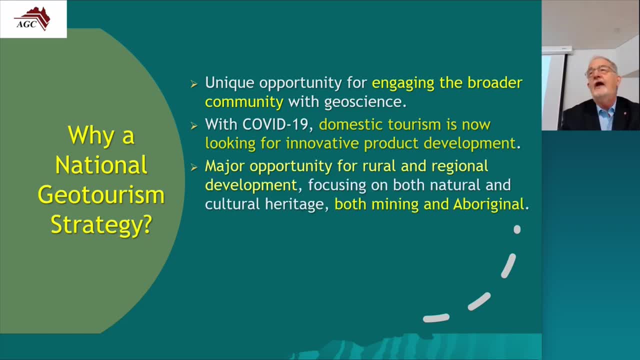 And that requires innovation in product development. And there's a major development opportunity for rural and regional communities focusing on both natural and cultural heritage, both mining and Aboriginal, And there's emerging grassroots community support around Australia interested in the whole concept of geotourism. 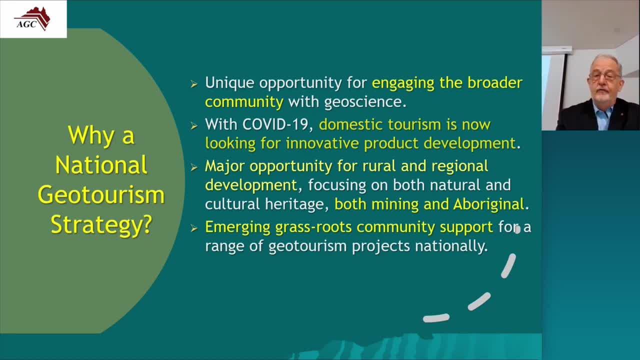 with some communities liking the idea to be able to aspire to develop geoparks, But in the meantime we're recommending focus on building geotrailers. So we need to gain the support of these projects by governments, And the government body that's responsible for that is the Geoscience Working Group. 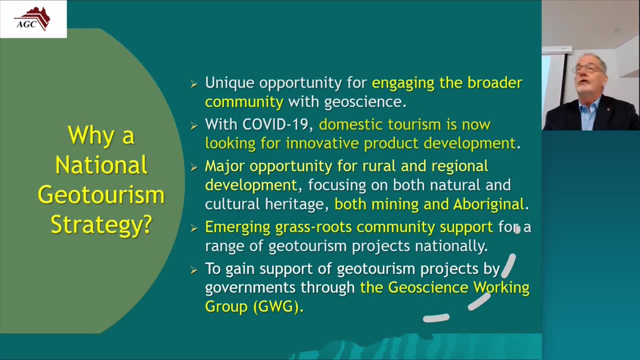 the GWG comprises the chief executives of the geological surveys in each state and territories, as well as the senior representative of Geoscience Australia. It's working with us to develop a process, And I'll say a little bit more about that in a moment. 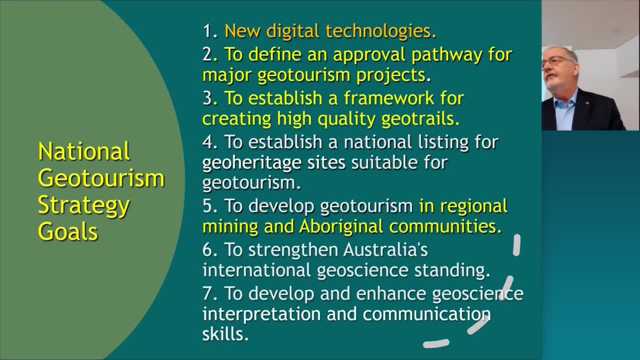 Now the strategy, and we developed these goals not in isolation, but in consultation with the geoscience community and in consultation with the GWG. The need for new digital technologies to define an approval pathway for major geotourism projects. We need a roadmap to enable companies and proponents to know how to get there. 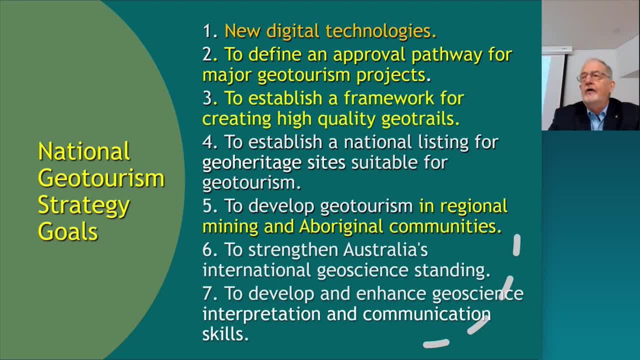 to establish a framework for creating high quality geotrailers. to establish a national listing of geoscience suitable for geotourism, because not all sites are suitable for geotourism, They need to be protected or they have access problems. 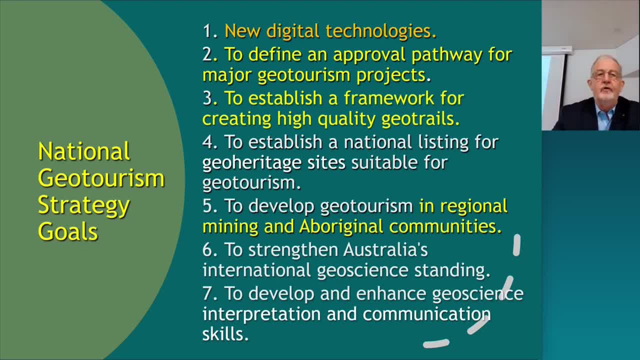 And to develop geotourism in regional mining and Aboriginal communities To strengthen Australia's international geoscience standing. that means to say anything we do create and promote by way of global geoparks- if we get there needs to be top quality. 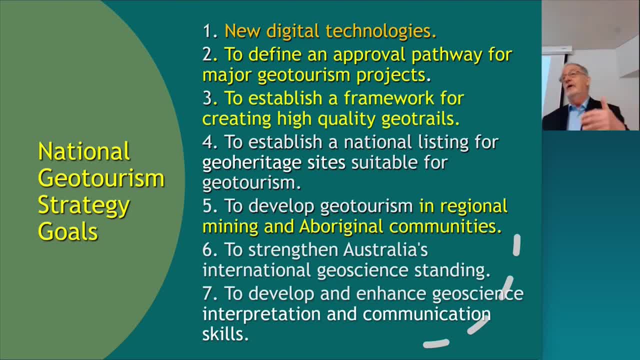 Australia can't be putting up second-rate product, given the geoparks elsewhere in the world are outstanding in the way they are presented and developed. And then to develop and enhance geotourism interpretation and communication skills, Particularly if a geologist is involved. 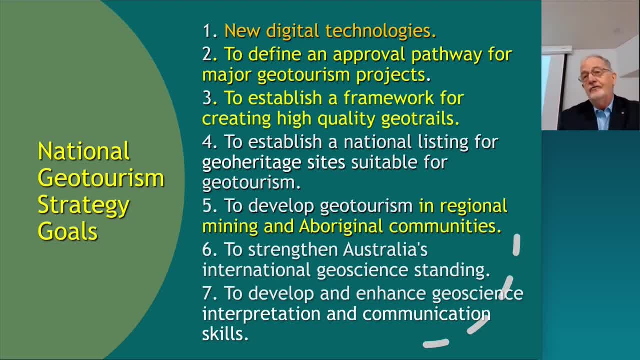 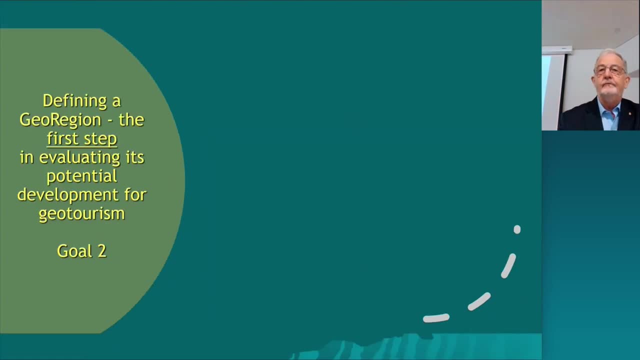 geologists and other people working in natural and cultural heritage need to be skilled to be able to get the message across, interpret areas correctly, And we're working with groups such as Savannah Guides to assist us in being good at that particular job. So they're the seven goals. 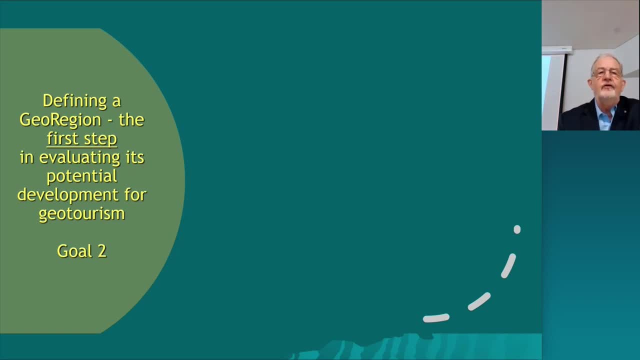 Now defining a geo region. Now, this is a concept we have developed, where we are suggesting that it can be an area defined by a proponent, Which might include, for example, a local government authority or a regional development authority having completed an approved 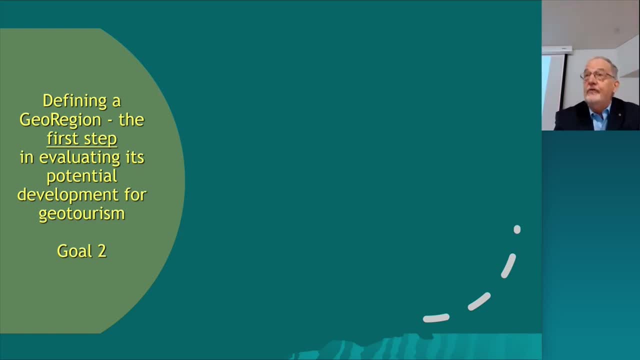 destination management plan based on geotourism principles. So before they even start getting their plans together, they actually look at what geotourism is about, And we have achieved this already in the Glen Innes Geo Region project in New England area of New South Wales. 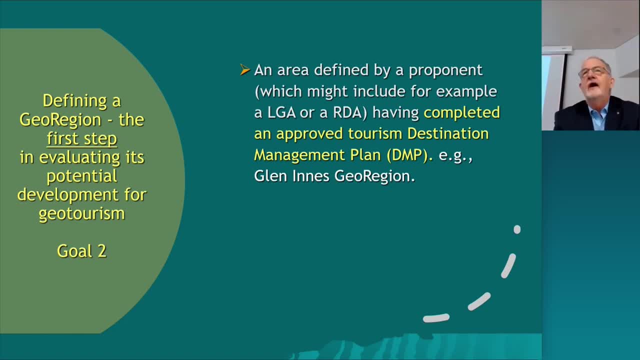 And then the proponent really needs to seek agreement from state government agencies, particularly the geological surveys, to see if an area is one has significant geoscience value- In other words, they get an expert opinion- But secondly, to identify areas of sensitivity. 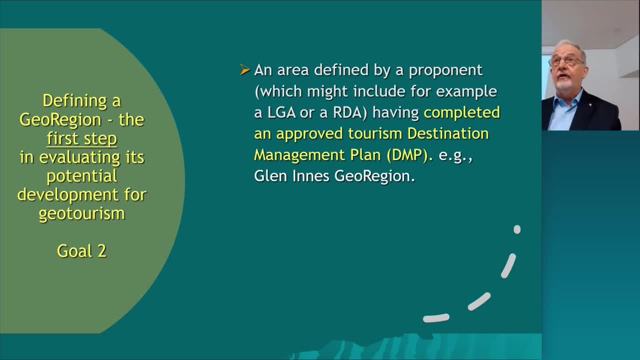 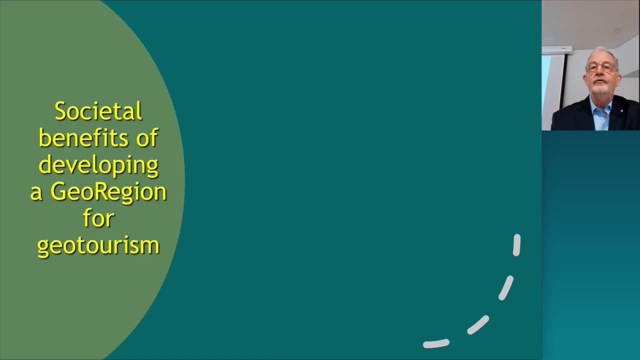 particularly in regards to exploration and mining access- Big, very big issue for the Australian mining industry. So this is kind of like. the first step we recommend is to look at what are the benefits of a georegion And then we can move on to what are the benefits of a georegion. 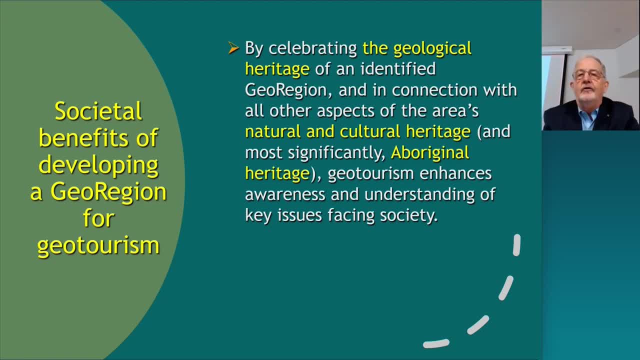 Well, we believe, by celebrating the geological heritage of that georegion and all the other aspects I've talked to, and natural cultural heritage, geotourism enhances awareness and understanding of key issues facing society, For example, again with climate change. 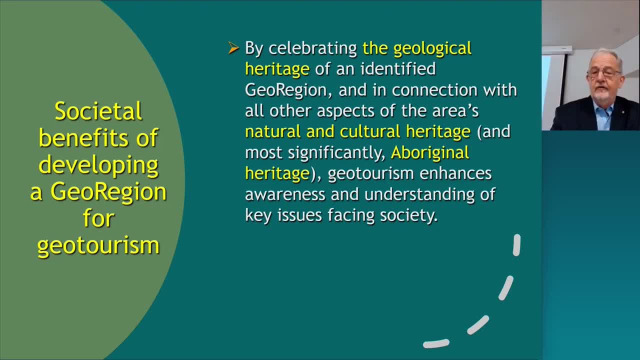 we've been able to demonstrate that in the Kuringai georegion Enable people to have a better understanding of the holistic nature of natural and cultural heritage, And it gives local people a sense of pride in an area and strengthens their identification with the georegion. 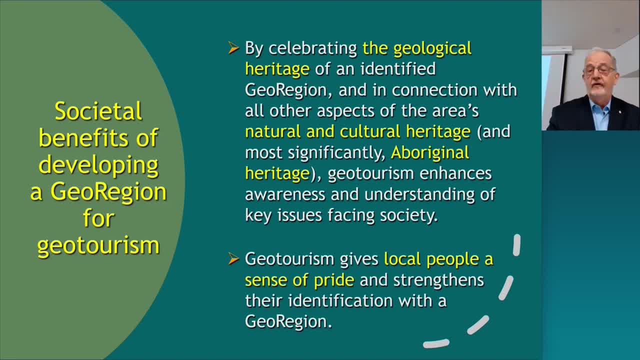 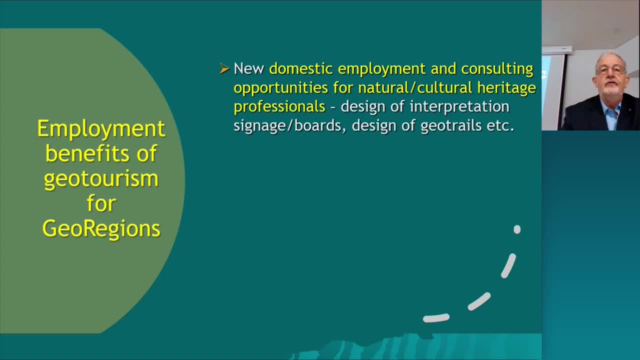 Communities like to be involved and that's one way they can make that step. What are the employment benefits? There's consulting opportunities for natural cultural heritage professionals, Again reaching one of the aims of the AGC: design of interpretation signage. 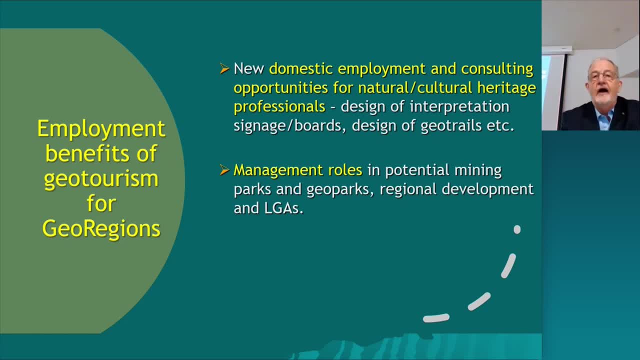 design of geotrails, management roles in national parks, other forms of areas working with local government agencies that do need expert support, And then, of course, the expected flow unemployment in tour operations and townships resulting from increased tourism visitation. 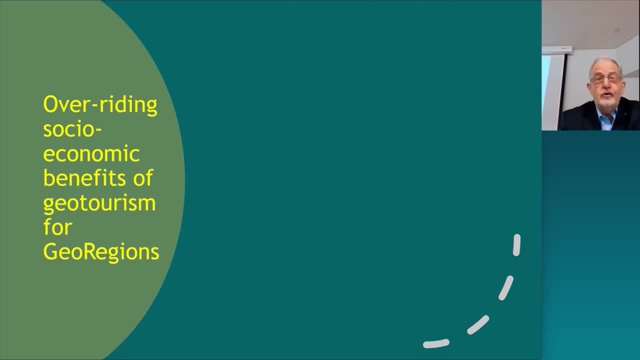 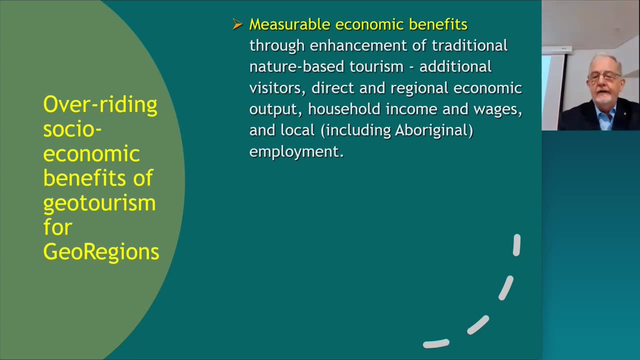 There, of course, overriding social echo- sorry, socioeconomic benefit- of geotourism for georegions. There's all the flow on multiply effects of tourism generally, which are well identified, but they can apply equally to geotourism projects. 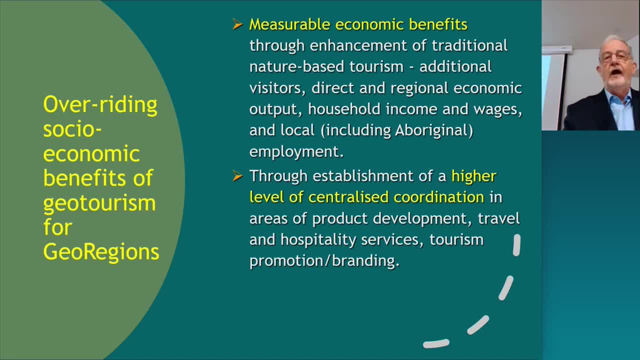 There's a better establishment of a higher level of centralized coordination. Australian tourism is terribly fragmented from area to area, state to state, and the lack of coordination is really making things not only difficult to develop but very confusing for the visitor. So the idea of decentralizing the coordination 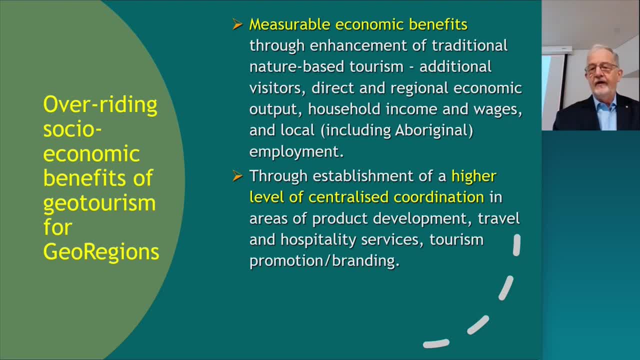 so that we're understanding working with the same brand and understanding how products can be developed which meets and gives credibility to the brand is important. So through this mission, community engagement is maximized and can be measured. So the role of the community in being part of this process, 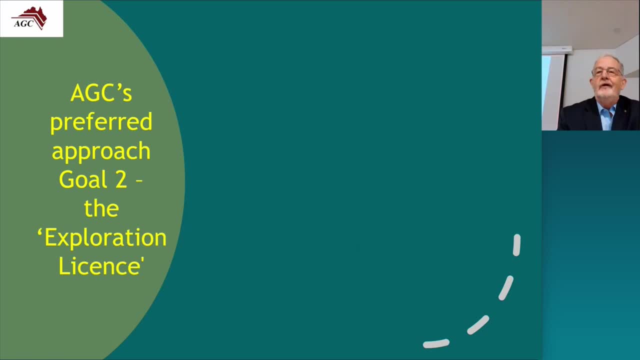 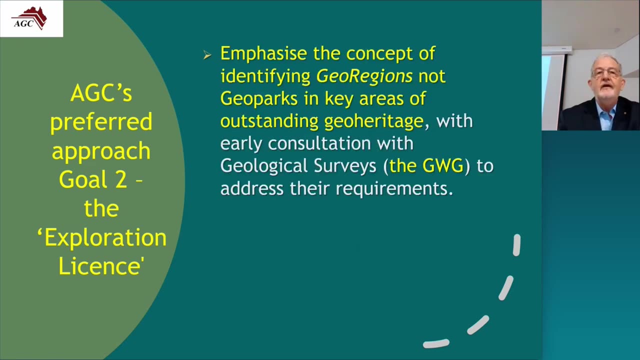 is very important. So we like the idea of the goal of creating this geo region approach because it's in a sense a exploration license, Like when a mining company comes into an area. they have an exploration process, They do the work with communities. 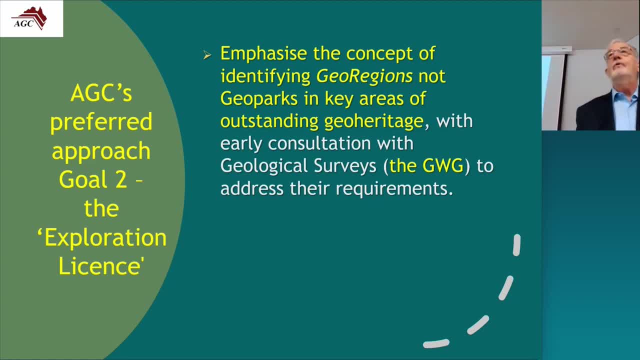 They do the exploration, They look at this, look at that, and there's no presumptiveness until they get to the stage where the government says: we would like you to build a mine and you'll need to do it because you've proved the viability. 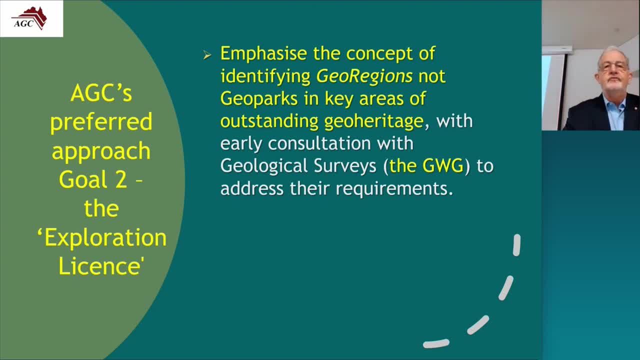 That's the same idea we're developing with the geo-region approach: Give the opportunity for consultation with state government, with the geological surveys, and that's why it's important we're engaging with the GWG to address their requirements. So by focusing on geo-trails as being that first easy step is an opportunity for the 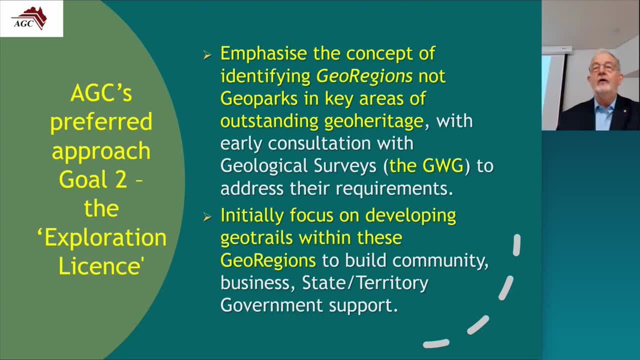 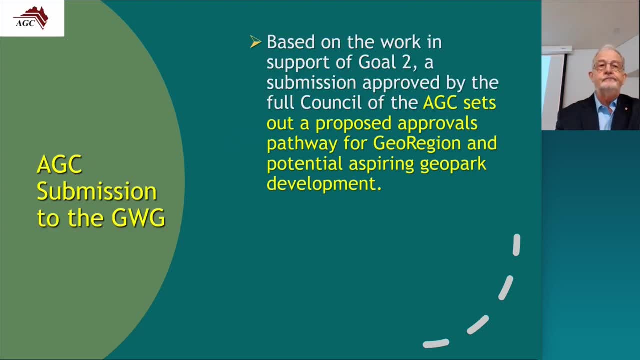 process to actually have some physical emphasis of how an area can be assessed and the extent to which that particular area meets visitor expectations. So at the present moment we've got a submission before GWG where the AGC sets out proposed approvals, pathway for geo-region and potential aspiring geo-park development. 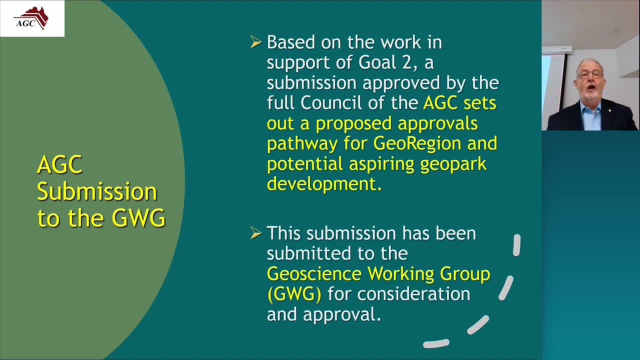 So we've got a plan. the government agencies through GWG are looking at it and hopefully we'll have a decision, hopefully in the next few months. It's been a long process But it's a very important. we get GWG support for what we want to do. 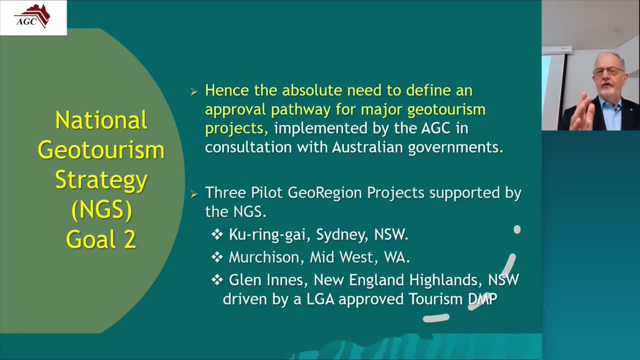 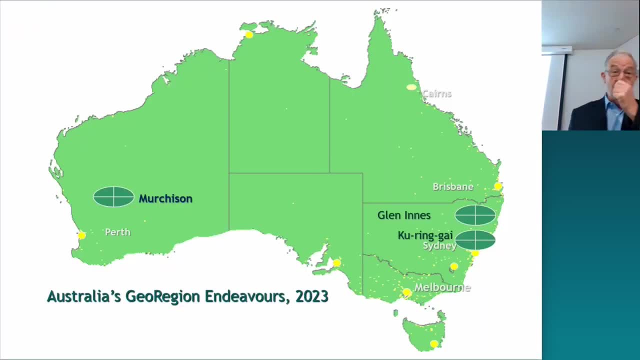 Now the strategy two talks about geo-trails, I'm sorry, geo-regions. We've got three projects active in Australia at the present moment and these are outlined in the west: the Murchison geo-region, the Glen Innes geo-region. I've spoken about that. 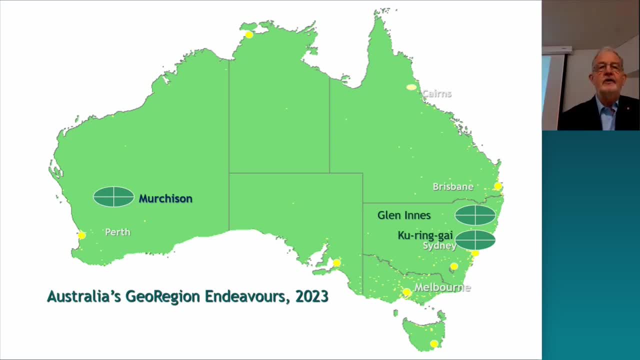 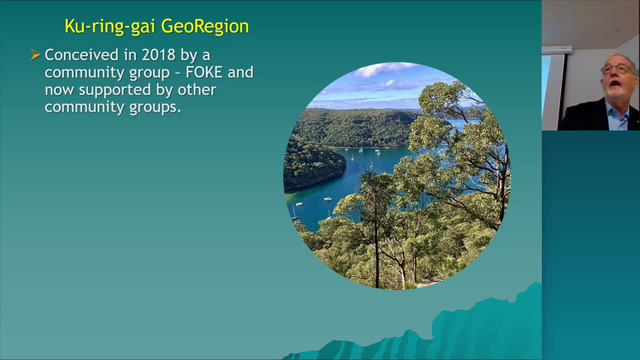 but also the Karingai geo-region. The Karingai geo-region encompasses land Inclusive of the Karingai Chase National Park, all the land right across to the northern beaches, from Barranjo South to DY. Now, that's an important project because it's been conceived by a local community group. 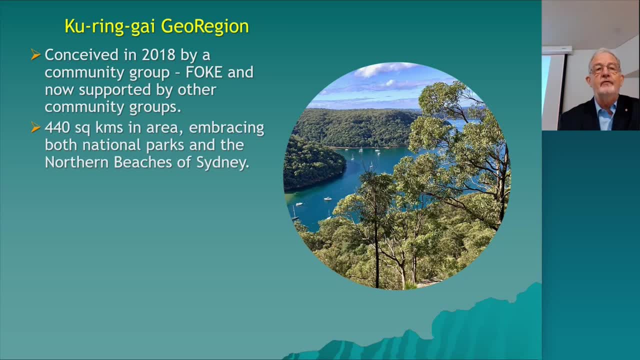 the Friends of Karingai Environment, supported by other community groups. It's only 440 square kilometres of area, embraces national parks, reserves, the northern beaches area, populated areas And the national park components about 50% of the area. 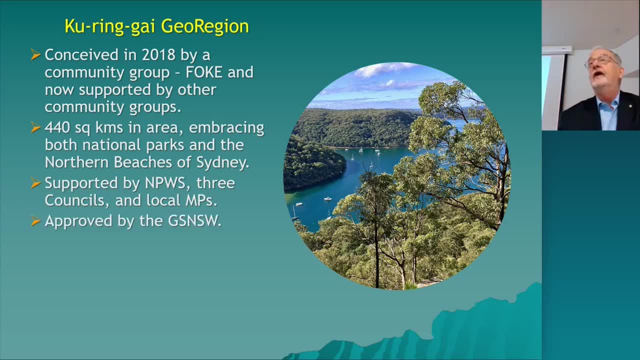 It's supported by the service, three councils, local MPs. it's approved by the Geological Survey of New South Wales, has no threat to exploration or mining in that area And we have recently completed a major natural cultural history document which outlines all the attributes and that's been published by the Linnaean Society of New South Wales. 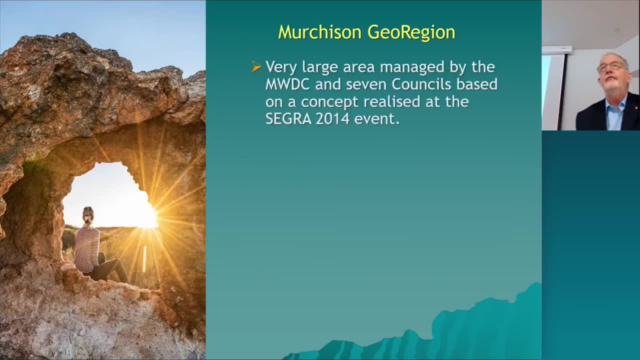 The Murchison geo-region is quite a different proposal. It's a very large area, over 100,000 square kilometres- and it's been managed by the Midwest Development Commission, which is a regional development authority and seven councils, based on a concept realised some years ago at one of our geo-tourism events. 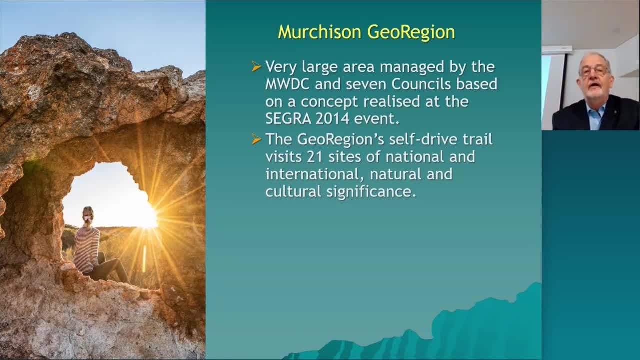 It's got a self-drive trail with 21 sites of national, international, natural and cultural significance. It's a journey. at the present moment, The potential geo-parking And the geo-park areas within that will have to be identified, discussed with the Geological. 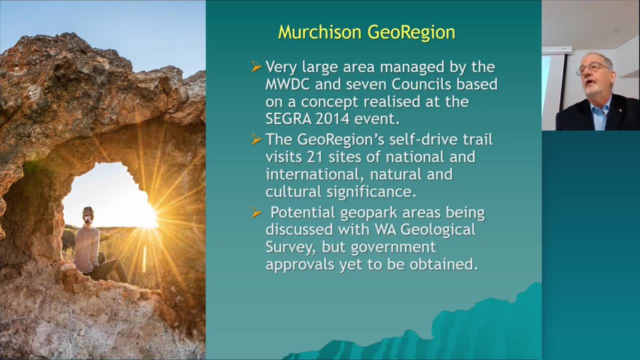 Survey and with Aboriginal people. So government approvals are yet to be obtained, but the people there are very keen to see some form of geo-park or other come out of this process, Though the technical access details for each of the sites also needs to be completed. 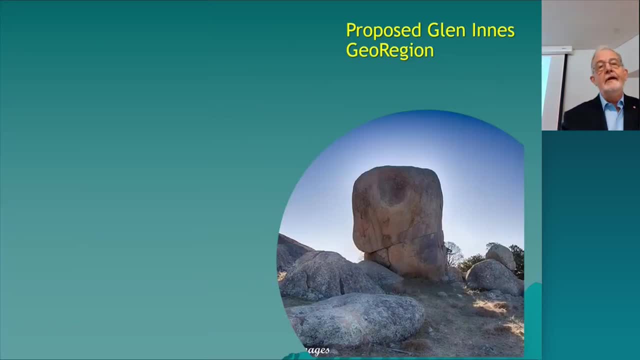 A big project, a lot of interest in Western Australia. The Glen Innes project which I mentioned has been approved by the Glen Innes Society of the Seven Council And it's driven not only by their particular destination plan but also by both regional 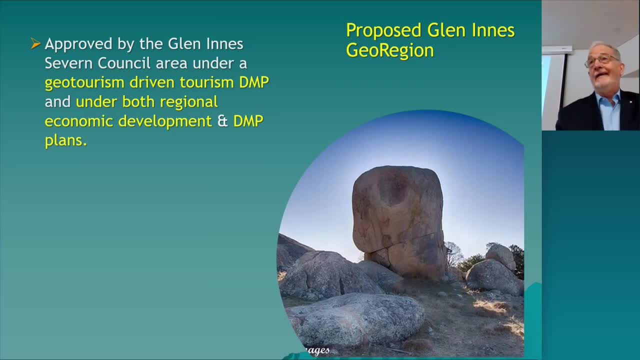 economic and destination management plan. So it's embedded in their planning mechanism and that's good because it's got, you know, support through various levels of government And it's been featured in a case study highlighted in the Austrade Thrive 2000,, which is a national tourism strategy project. 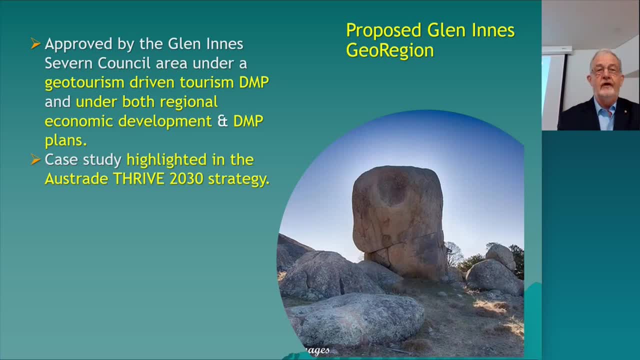 It's a great opportunity for geotourism and I'll explain that in a moment. It's called Natural Cultural Heritage Order Completed. So they've done their homework and they've got funding approved for various geo-trails and a major rail trail, all working within the concept of a geo-region. 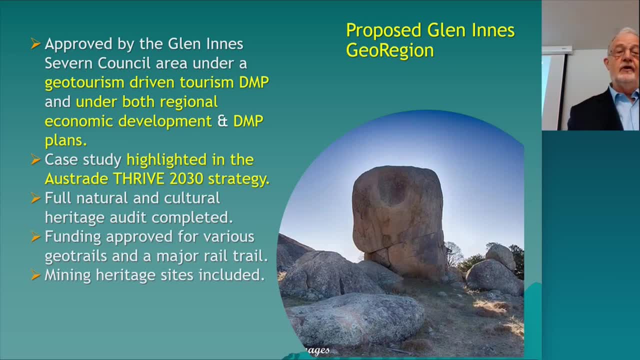 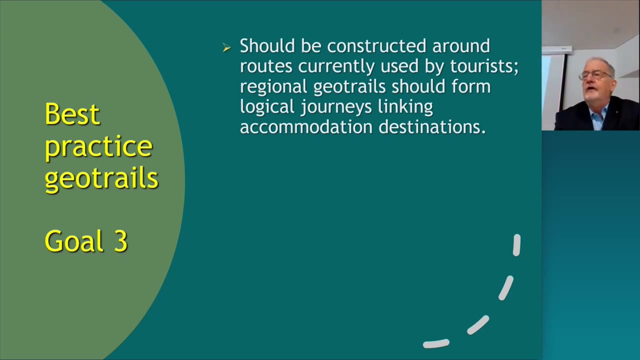 And, importantly, it has a large amount of mining heritage sites included within it Still awaiting approval from the Geological Survey of New South Wales Registration. Just turning to geotrails, as I mentioned, they should be constructed around routes where relevant are used by tourists. 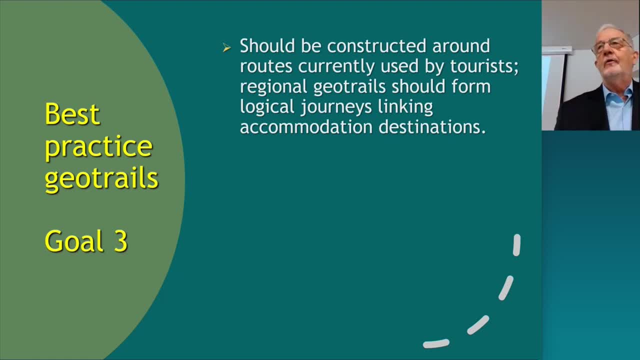 The regional geotrails should form logical journeys linking accommodation destinations. If you're looking at a localised area, you might have a set of geosites over a small area. A geotrail links them and tells a story, And it has to be a cohesive story so people understand the logic of the of the geotrail concept. 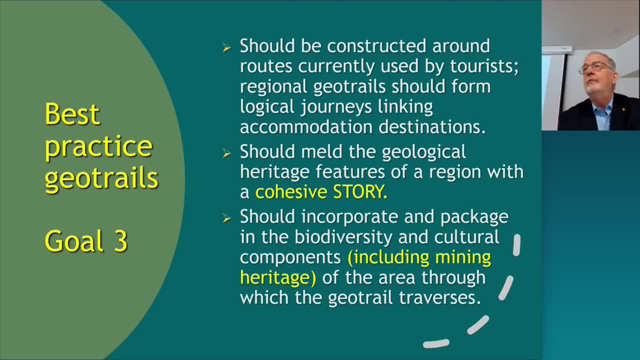 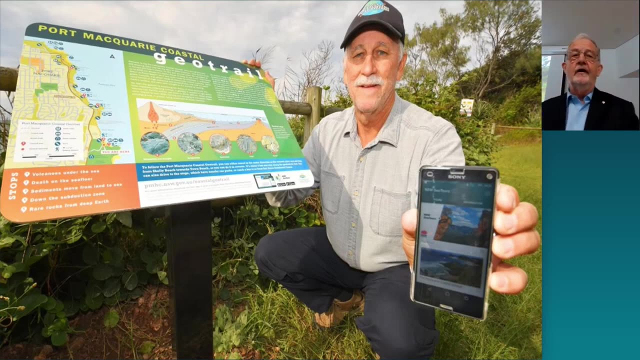 And it should incorporate, where it is available, packaging, the biodiversity and cultural components, including mining heritage, of the area for which the geotrail traverses. Now, one of the successful local geotrails was developed several years ago at Port Macquarie, along the coastline. 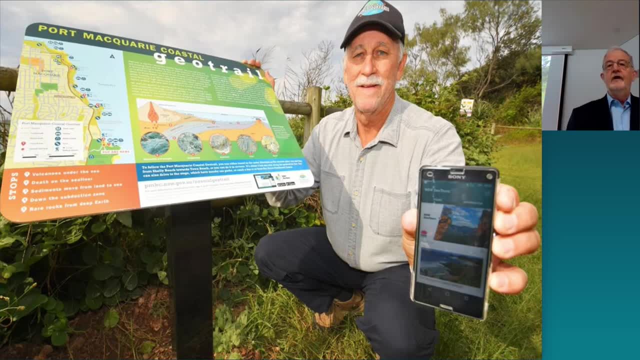 So in that particular case, the collaboration of Newcastle, the council, Newcastle University, local council, National Parks and Wildlife Aboriginal groups put together this four kilometre geotrail. You have signage and also supported by a smartphone application. So that's the sort of thing that can be done And that was interestingly. 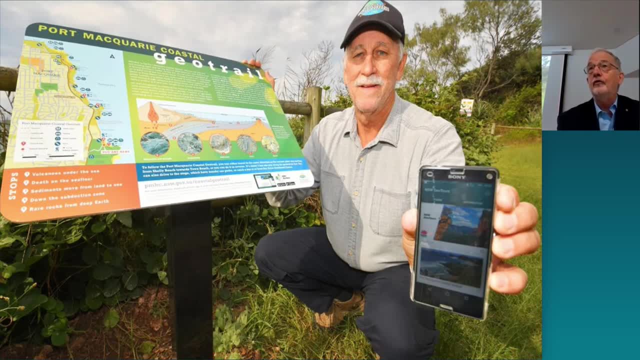 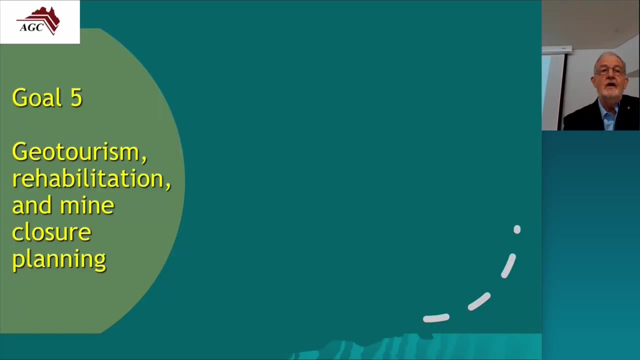 its biggest benefit has provided a resource for school groups to come down and have something in the field to look at. So that's been the wasn't realised When it was designed, But that's what's happened. The teachers love it. We should keep that in mind when we're thinking about other geotrail development. 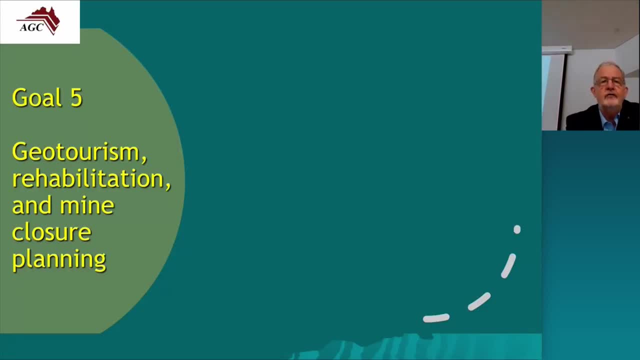 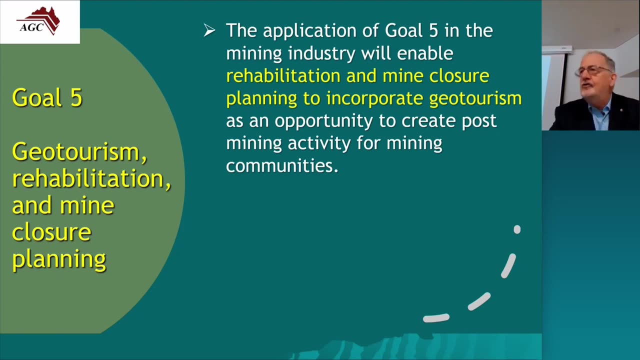 Now, goal five is an important goal because it talks about geotourism being part of rehabilitation and mine closure planning. We believe that the application of this goal- that's, looking at the way of incorporating mining and Aboriginal interests into projects- will help in the rehabilitation mine closure. 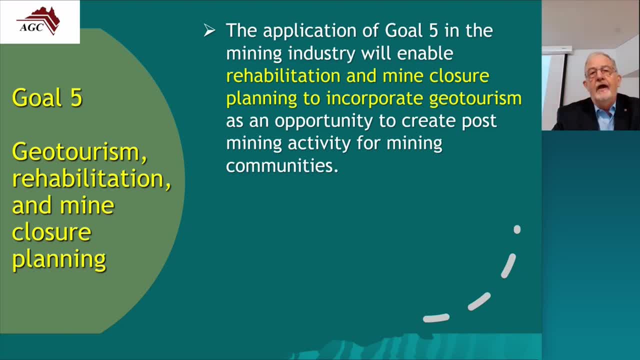 planning process and an opportunity to create post mining activity for mining communities. In other words, if mining companies get involved in issues relating to mining heritage and rehabilitation. thinking about mine closure, they're also thinking about what happens when the mine closes, And now we're working on that concept through the AUSIMM's social environment committee to have geotourism being part of the mechanism that companies ought to look at. 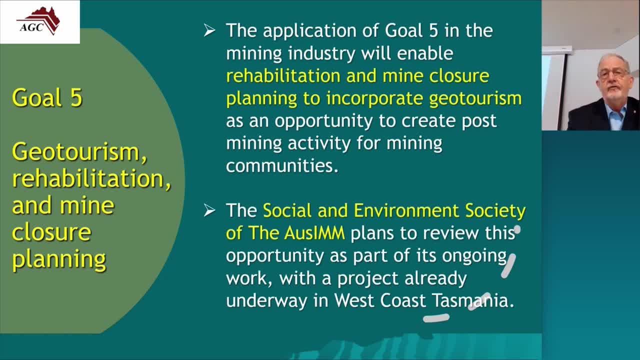 And that's what I've mentioned. And that's what I've mentioned there, And we already started this project with an ongoing work, with a project underway in the Hercules mine site in Rosebury, West Coast, Tasmania. Geotourism work has started. 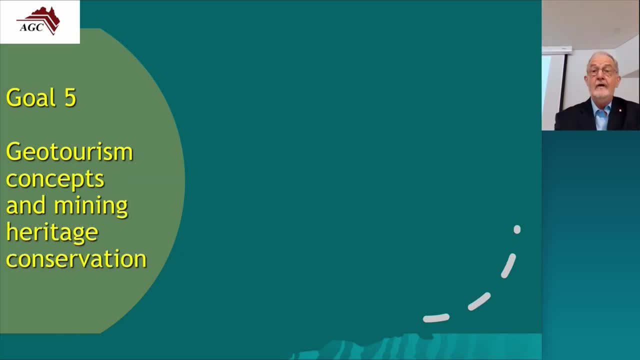 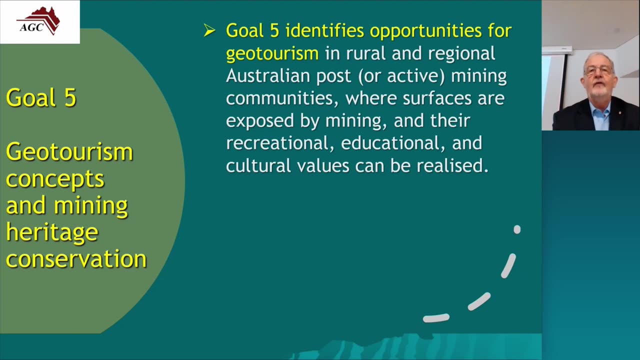 It's been mapped out and the company is looking at what they can do, So we see that. goal five identifies opportunities for geotourism in rural and regional Australia where the surface is exposed by mining, and their recreational, education and cultural values can be readily realised. 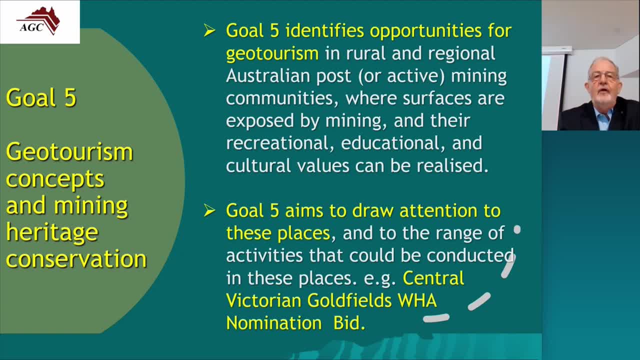 We aim to draw attention to these places in the range of activities that could be conducted. For example, we're now working with the Central Victorian Goldfields World Heritage nomination bid, where they're agreeing to use geotourism as the driver and in turn will provide the geological mining heritage advice that they can build the case for their particular nomination. 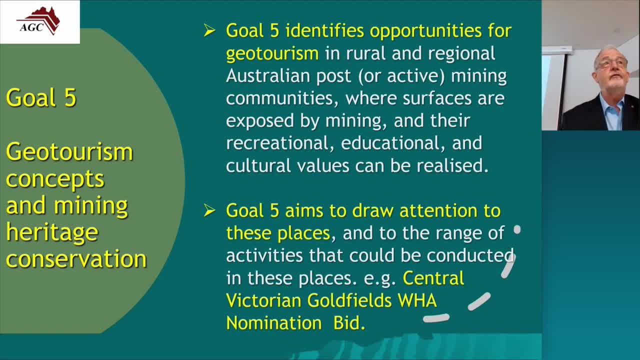 It's an example of what can be achieved. We believe if that is a success, other areas in Australia will say: gee, that works well. We can see how geotourism can work and they'll pick it up. In that sense we hope it will lead to other projects around Australia. 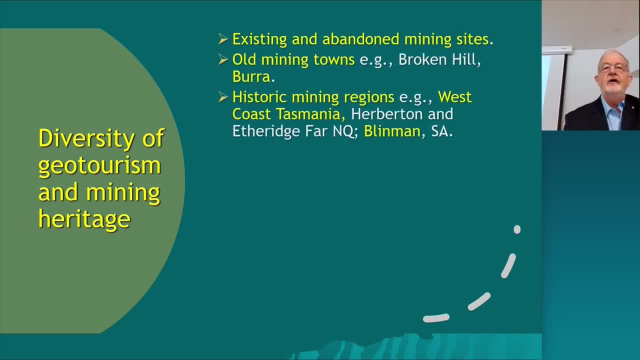 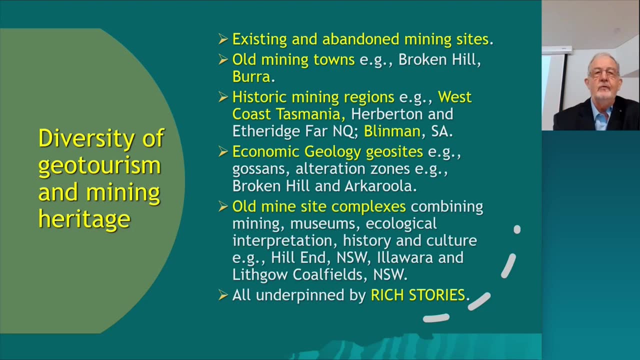 Of course, there's a whole range of diversity in mining sites around Australia: Regions, mine sites, geosites, old mine sites, complexes- all underpinned by rich stories And, by and large, most of which are not incorporated into the traditional geotourism product. 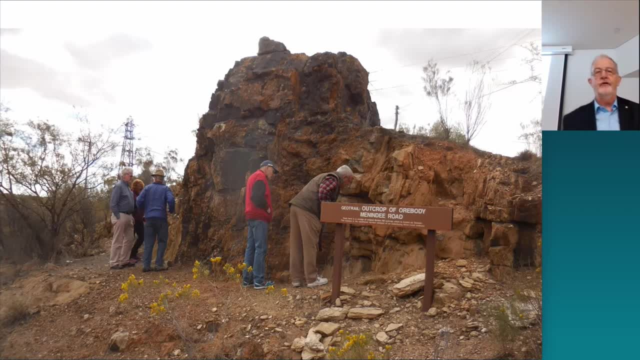 We hope that we'll be able to do that. There's an example of those geologists again at the important geotrail site at Broken Hill, the Gosselin. That's an important part of the economic geological geo heritage not well identified in Australia. 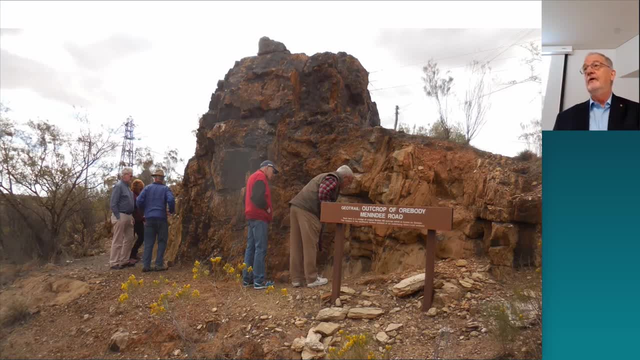 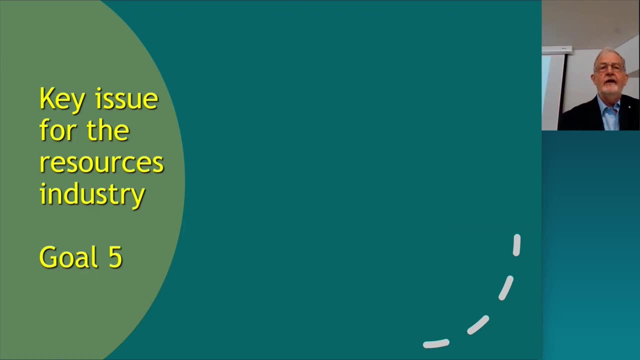 but it does need to be done because those sites are important for future economic development, as well as being able to tell the story about those mines. Now, the key issue we believe for the resource industry in Goal 5 is acknowledgement of Aboriginal cultural heritage. 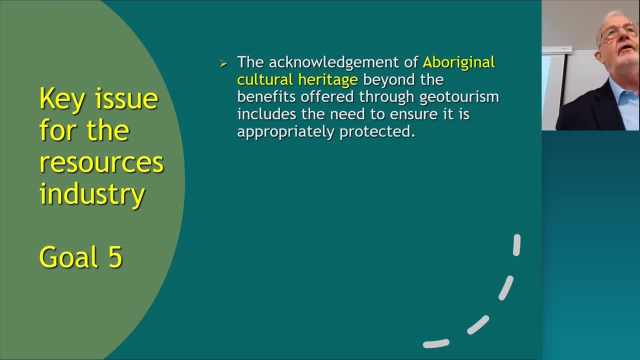 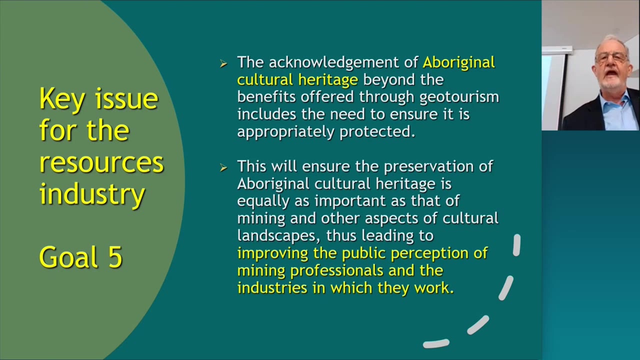 beyond the benefits offered through geotourism, including the need to ensure it is appropriately protected. Think about the experience last year with the Rio Tinto Dugan Caves situation. This will ensure the preservation of Aboriginal cultural heritage is equally as important as that of mining. 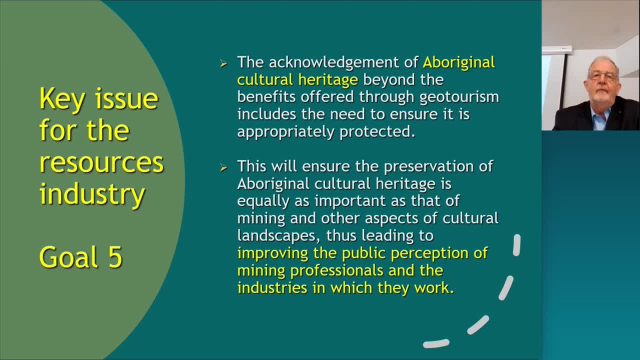 and other aspects of cultural landscape, thus leading to improving the public perception of the work of mining professionals and the industries in which they work. The last thing we want is for our profession to be considered to be environmental wreckers and people that don't understand the needs of Aboriginal culture, etc. 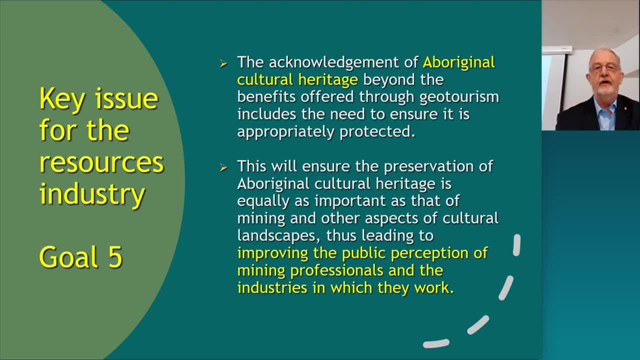 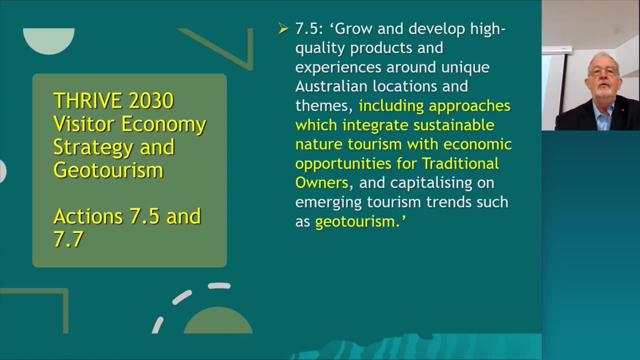 So this is a key issue that we're working on through that particular strategy. Now I mentioned the FRIVE 2030 visitor economy strategy and geotourism. Well, that reads: grow and develop high quality products and experiences around unique Australian locations and themes. 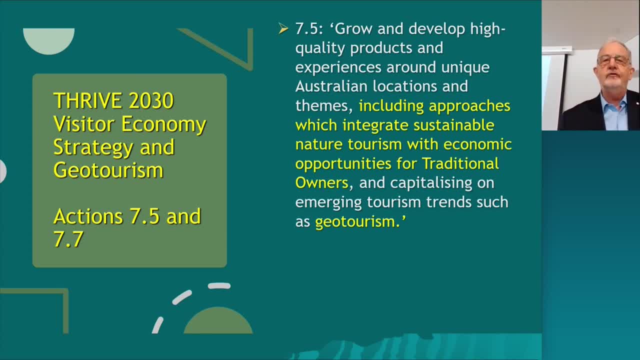 including approaches which integrate sustainable nature tourism with economic opportunities for traditional owners and capitalising on emerging tourism trends such as geotourism. We said hooray. Geotourism has been recognised by the tourism industry and we have an action ascribed, endorsed by government, to do something about it. 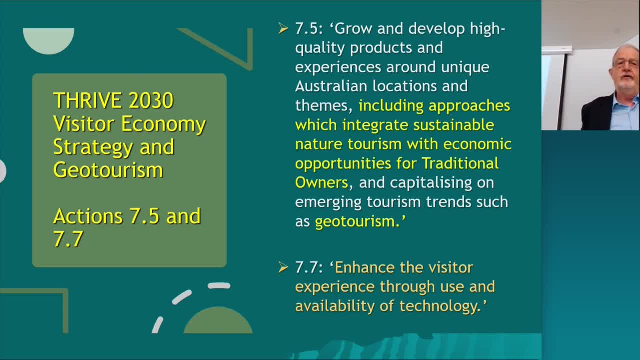 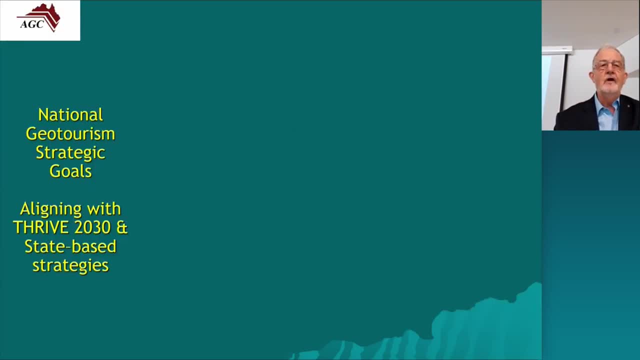 This is great. Also, they had another one which related to the experience for use and availability of technology, and I'll show the importance of that in a moment. So when we look at the new digital technologies, whether they be 3D visualisation, augmented and virtual reality, cutting edge work. 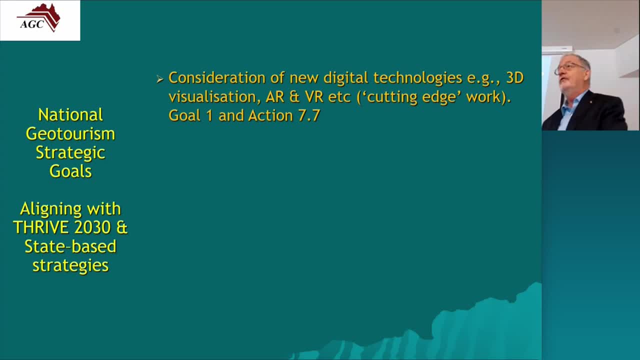 our goal one and the Action 7.7 line up, So we've got an opportunity as an industry sector to show the tourism industry generally. we're at the cutting edge And a lot of work's being done in Geoscience Australia and various universities around Australia. 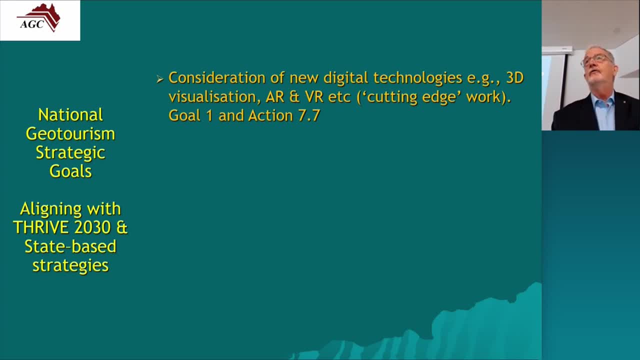 augmented reality where we can be able to show the rest of the tourism industry how those technologies can be applied through the geotourism approach. We think the improvement of the new pathway for major geotourism project talks that's goal two and Action 7.5 work together. 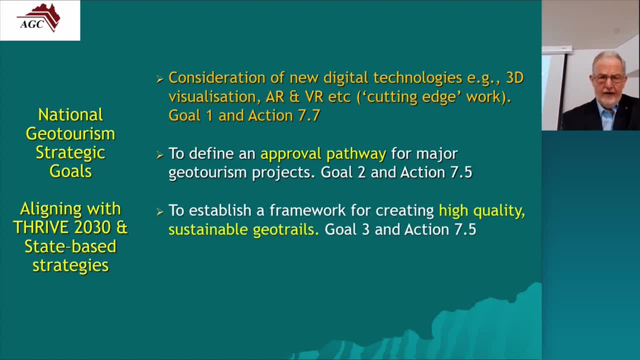 And we think the framework for creating high quality, sustainable geotourism is part and parcel of the delivery of Action 7.5. And to develop geotourism in regional mining and Aboriginal communities. goal five and Action 7.5 are lined up in a scenario in which we can take a degree of responsibility. 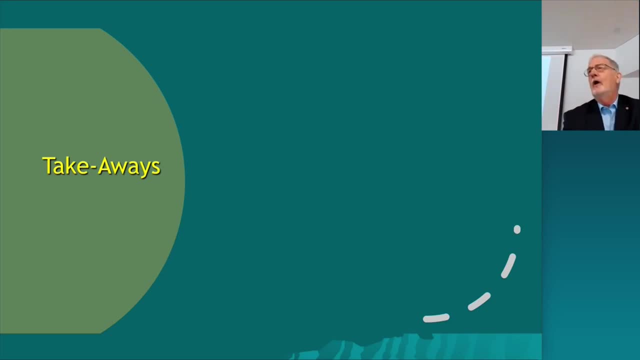 and ownership. So the takeaways to my presentation today are these: Geotourism is increasingly being recognised worldwide as a major deliverer of nature-based tourism. That is undeniable, And it's important to recognise that the countries which are preeminent in the development of geotourism and geoparks 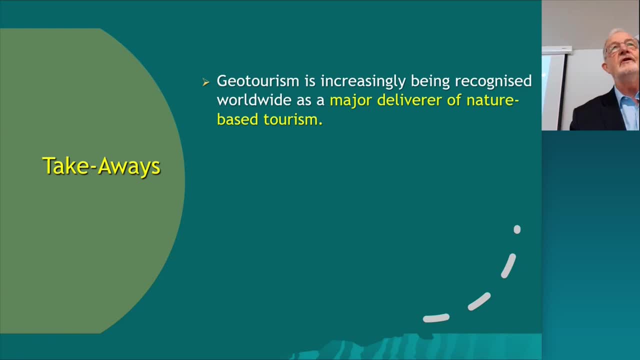 countries like China, Indonesia, a good part of Europe, just as a case in point, 46 countries are bringing tourists to this country And they know what geotourism is about. They know what geoparks are about, So we've got to have product there that meets their needs.